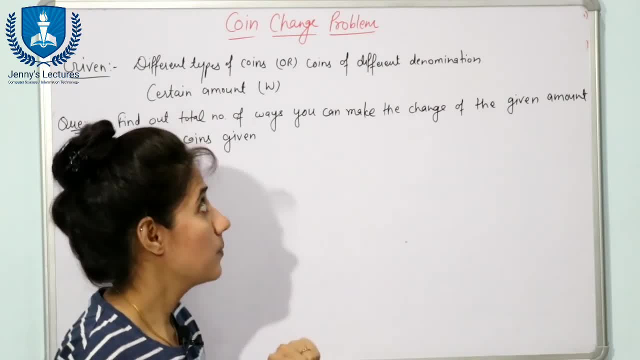 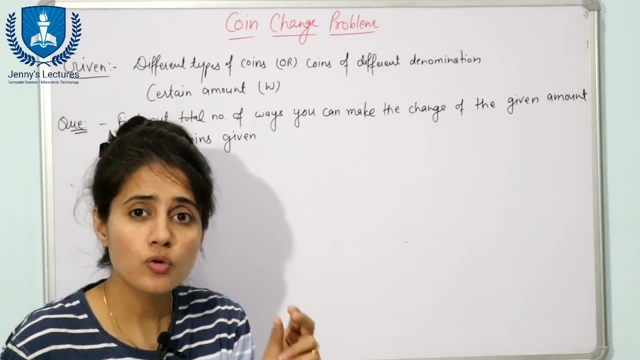 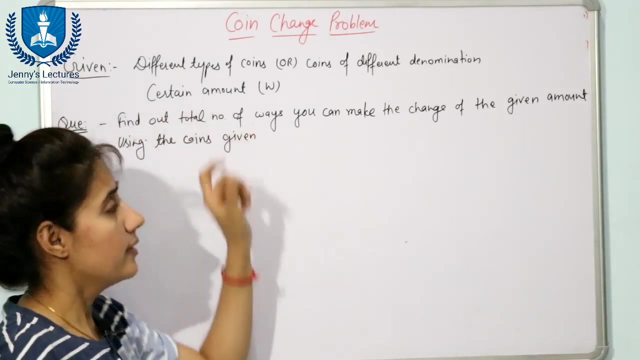 next video. fine. so the problem is you are given different types of coins, or you can say coins of different denominations, like one rupee coin, two rupee coin, five rupee coin, ten rupee coin, ten rupee coin, something like this, and you are given a certain amount. fine, now the 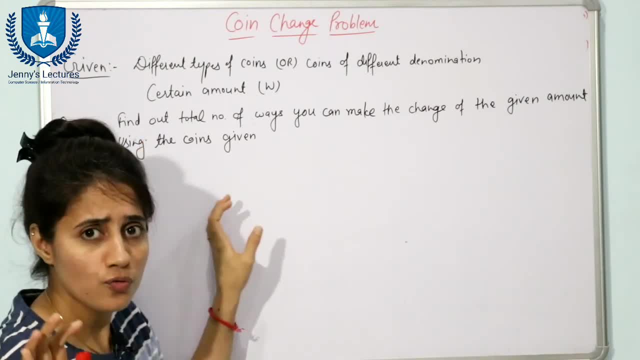 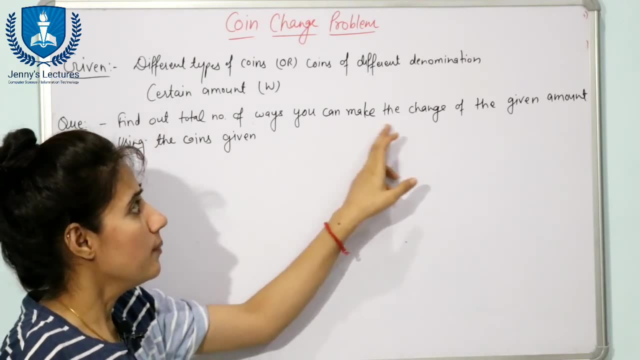 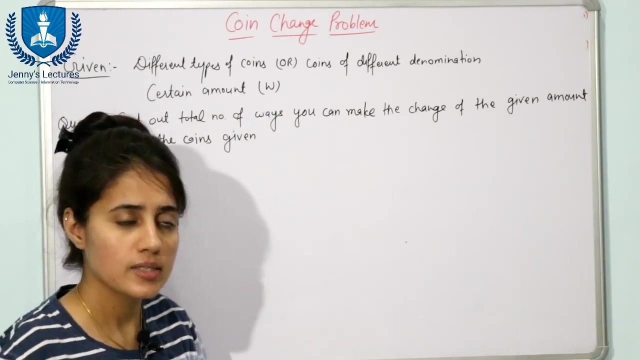 question is, or the problem is, you have to find out in how many ways- or you can say the total number of ways- you have to find out in which you can make the change of the given amount using the given coins. see, let us take one example. coins are given. 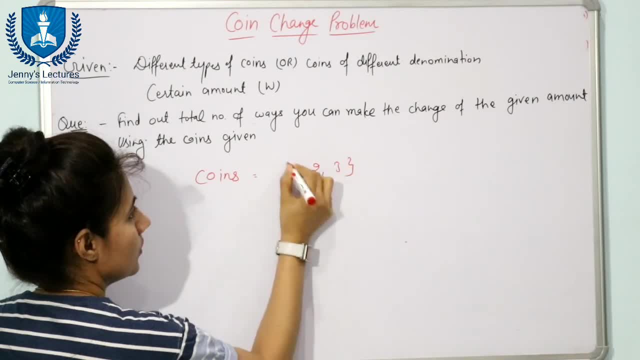 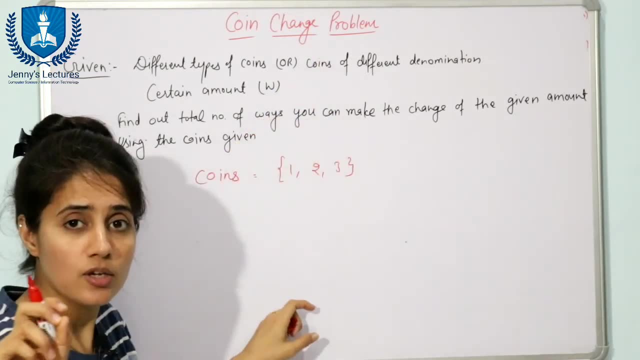 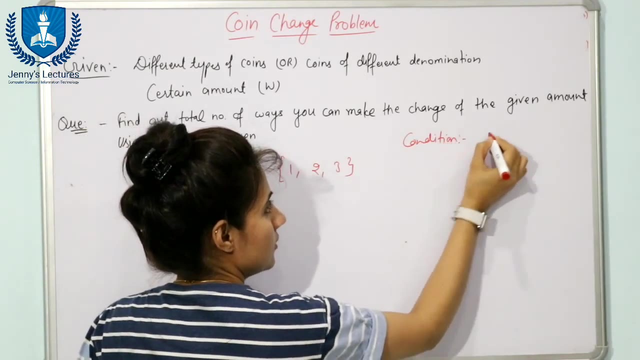 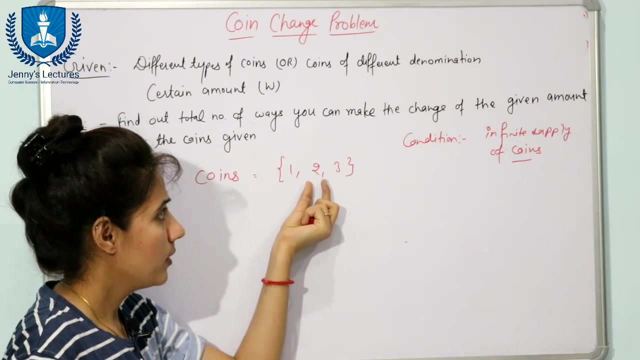 you have one, two and three, denomination of one, two and three. and here, here see, the condition is you have infinite supply of coins. that is very important. here the condition is infinite supply of coins. you have fine denomination of one, denomination two, denomination three. you are having coins of these denomination and the amount given is 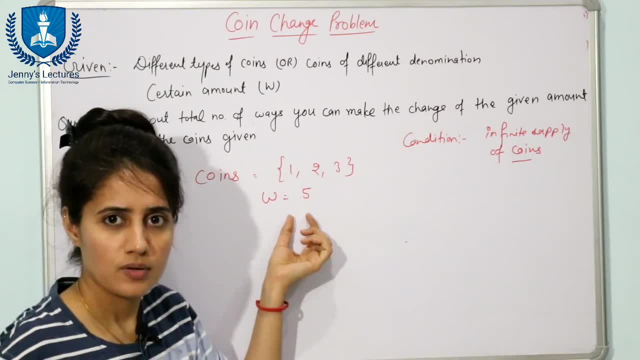 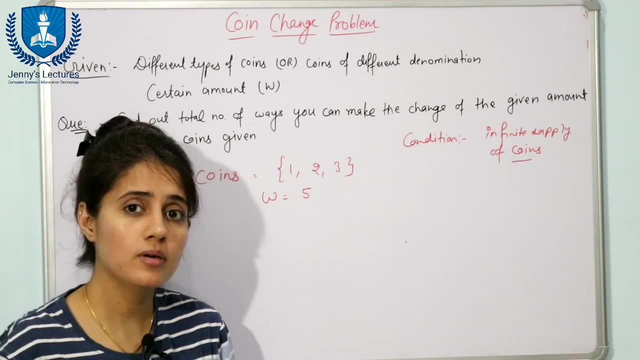 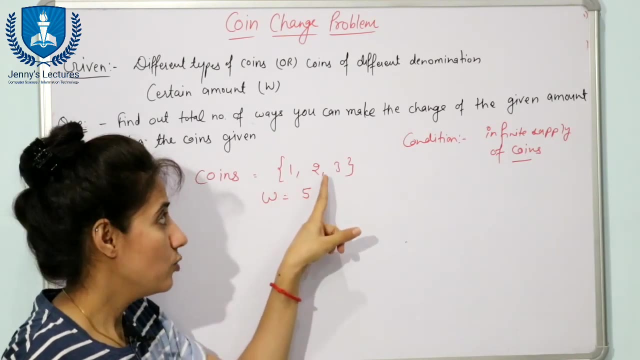 one and you have five. let us take an example: you went to a shop and you maybe bought something and in return, in return, maybe a shopkeeper has to give you five rupees, but he is not having a five rupee coin, he is having only one rupee coin, two rupee coin. and see, although 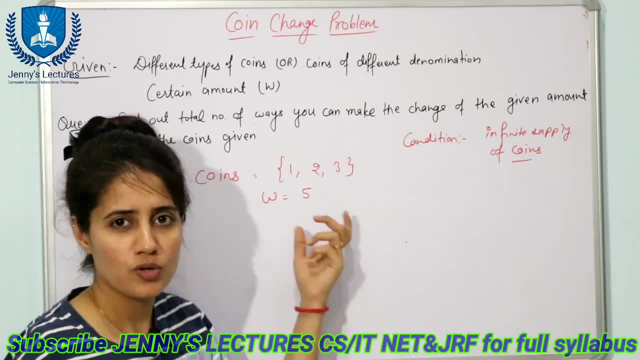 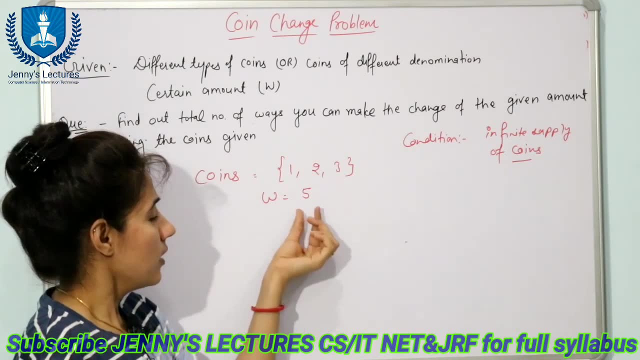 practically it is not possible to have three rupee coin, but when we are solving these type of questions then we assume we have one rupee coin, two rupee coin, seven rupee, ten rupee and something like this. fine, now how he or she is going to solve this type of problem. 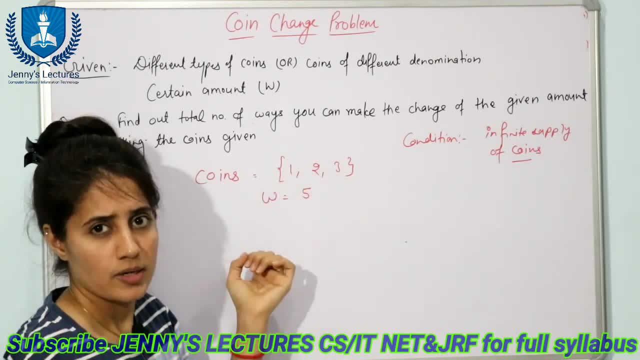 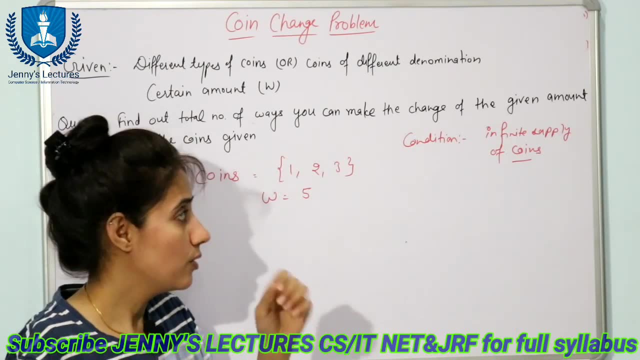 right. so now, here we have five rupees coin, five rupee coin, eight rupee coin, nine rupee coin. can give you five rupees using these coins, and the condition is he is having infinite supply of coins. so first, first thing is he can give you five, one rupee coin. that is fine. one, one, one, one and one. 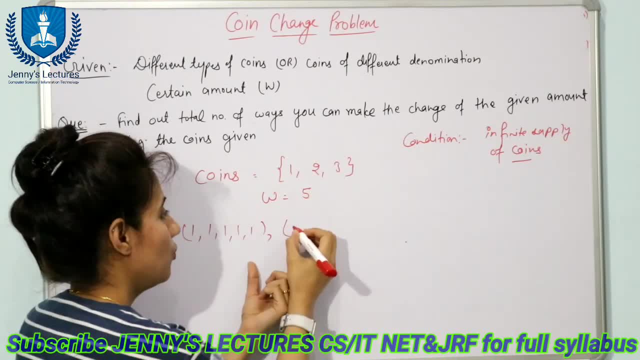 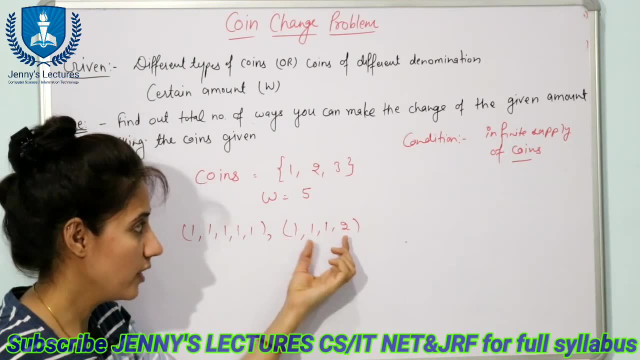 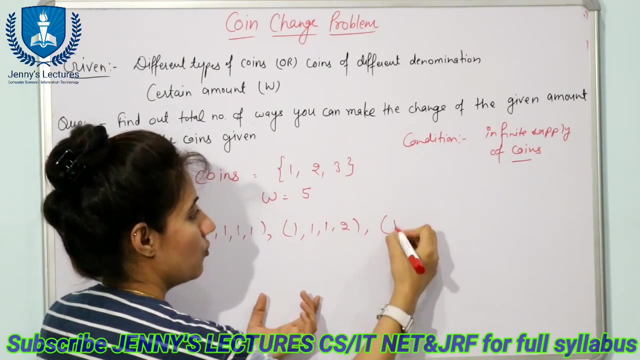 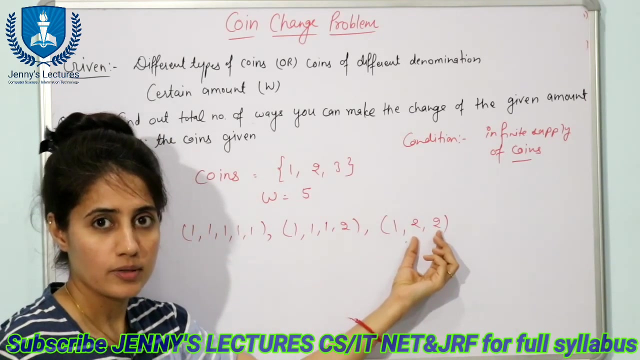 or second way is he can give you three one rupee coin and one two rupee coin. the total is five. two, one, two, three, four, five. that is also fine. or third way is he can give you maybe one one rupee coin and two two rupee coin. that is also five that this. this also makes a total of five, two plus two. 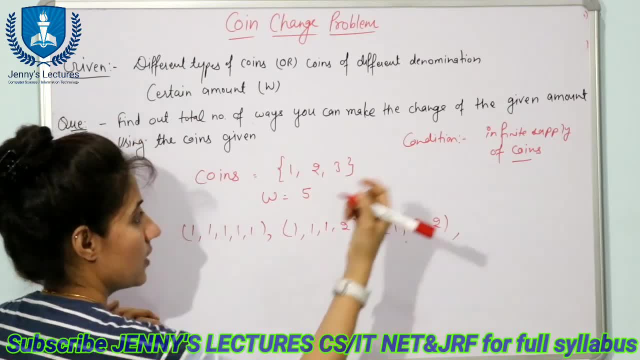 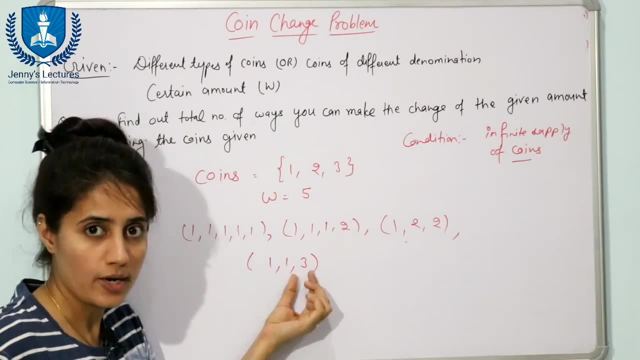 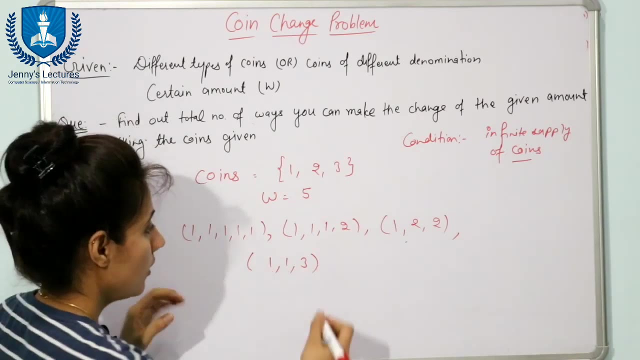 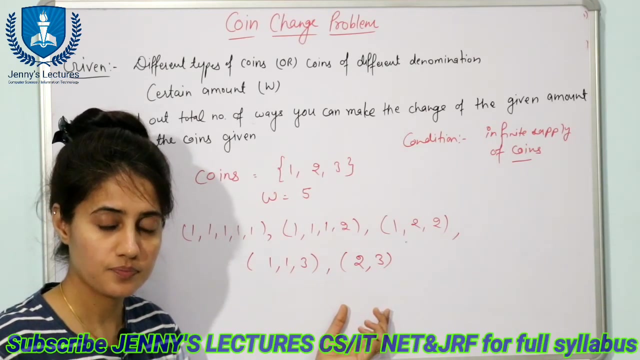 plus one, that is five. or another case is maybe he can give you one, one, two, one rupee coin and one three rupee coin. that is also fine, will make a total of five, three plus four plus one, that is five. or another way is maybe he can give you one two rupee coin and one three rupee coin. now i guess there is no way he. 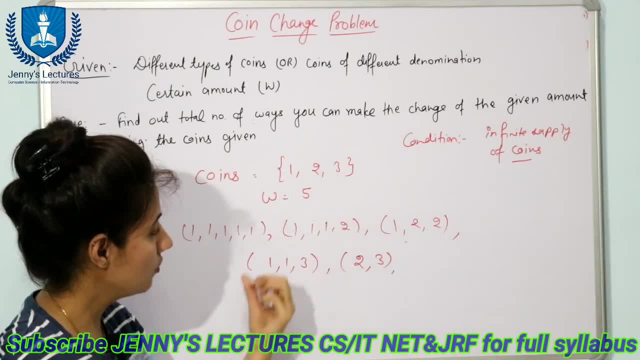 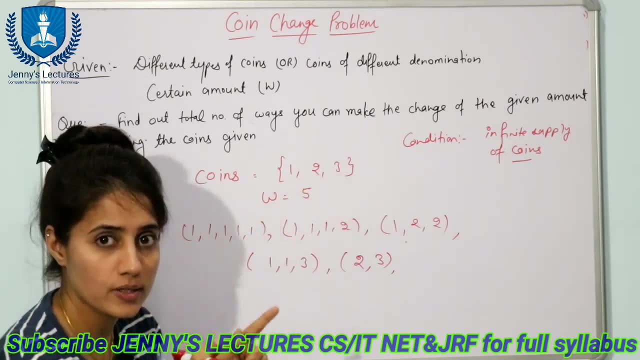 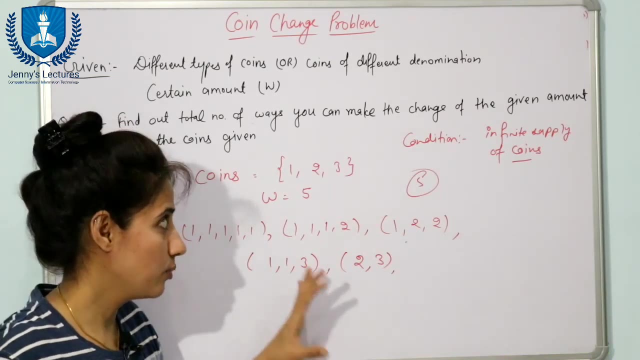 can give you these coins to make a total of five. so total ways are total ways to make this sum using these coins says one, two, three, four and five ways. now we will solve. we will take one more example and we will solve that problem using dynamic programming. 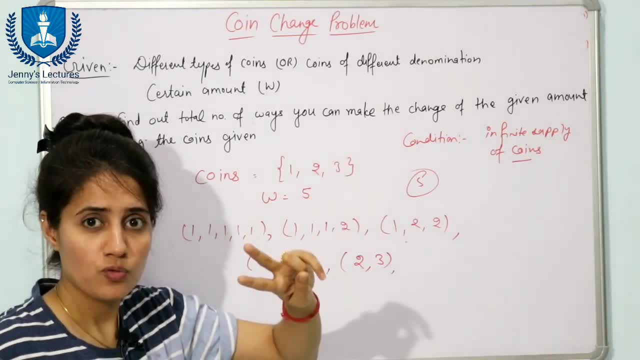 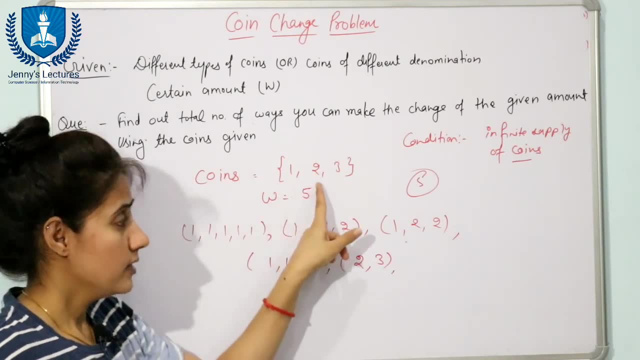 see, one is this kind of problem. i have already told you there are two types of coin change problem. one is this kind of problem. you have to find out total number of ways. second problem is coins are given. different denomination of coins are given. certain amount is given. you have to find out the. 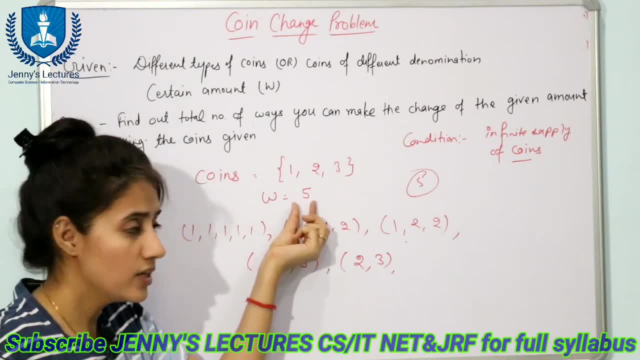 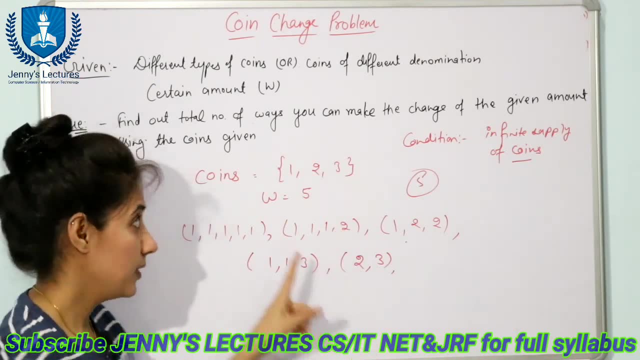 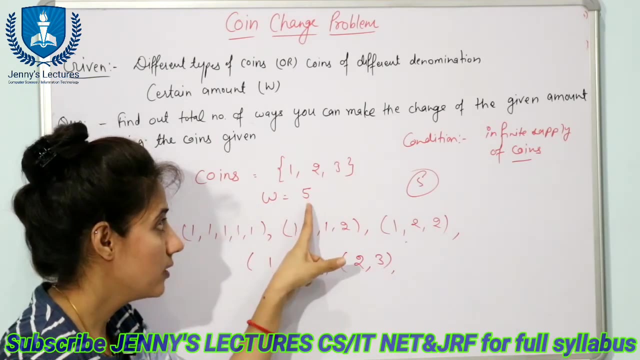 minimum number of coins to make this, this amount, using these coins. so if if we'll solve that problem now, let's consider this same example. then suppose coins are one, two, three, total is five. now you have to find out the minimum number of coins to make this sum. now, if we choose this set, 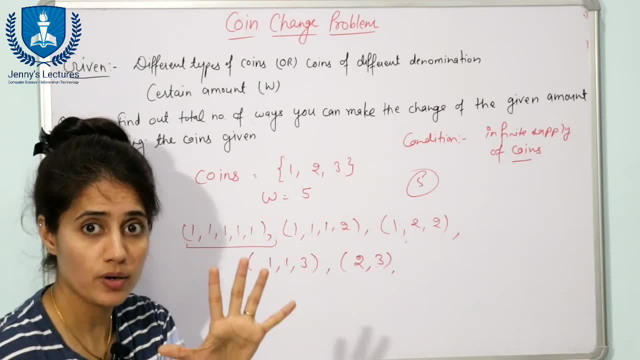 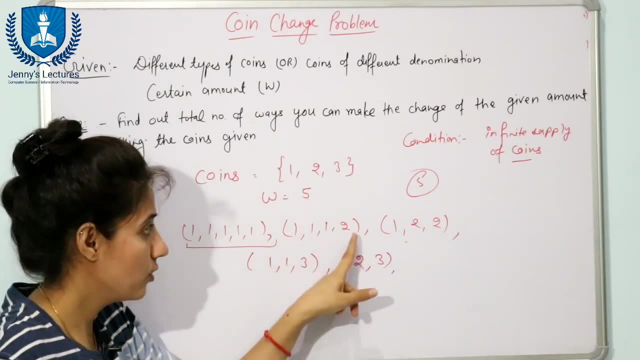 then how many coins we need to make this: five, one, two, three, four, five, five, one rupee coin. fine, if we choose this way, then how many coins you need to make a sum of five: one, two, three, four, four coins: three, one rupee coin and one two rupee coin, something like this: 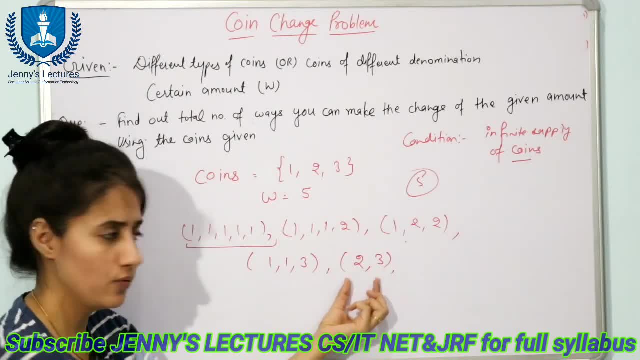 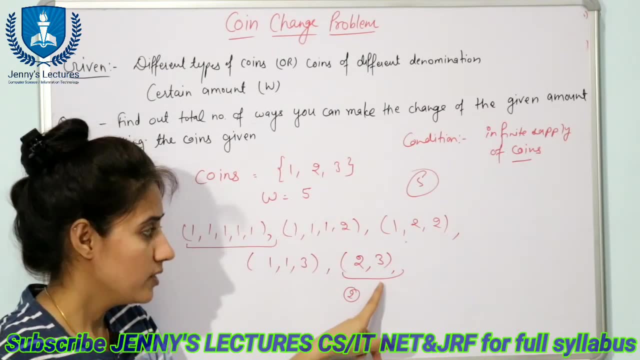 these ways. minimum number of coins are this one. if you choose this, set two coins, you need to make this total. second problem is something like this: you have to find out minimum number of coins, but in this video i am going to tell you how to calculate the total number of ways. 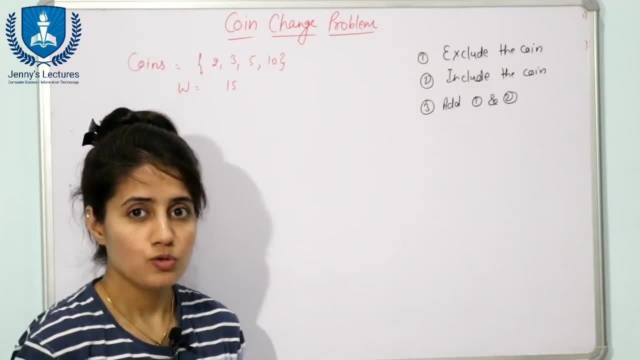 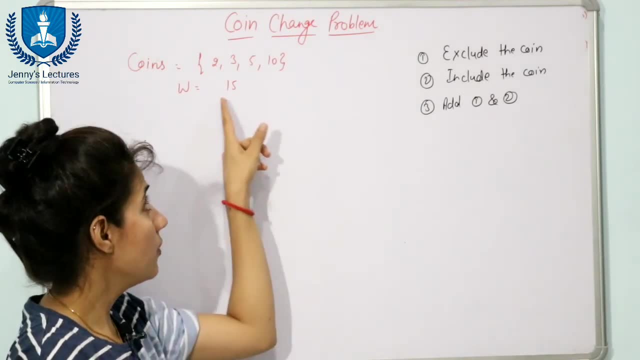 in next video, we will discuss how to calculate minimum number of coins. so let us take this example. we are given this coins of denomination 2, 3, 5 and 10, and the amount given is 15. now you have to find out the total number of ways in which you can make a change of this. 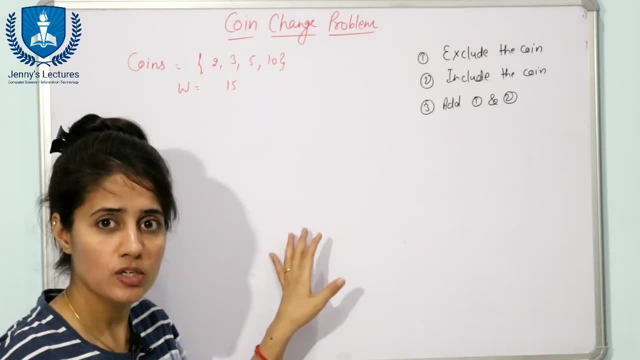 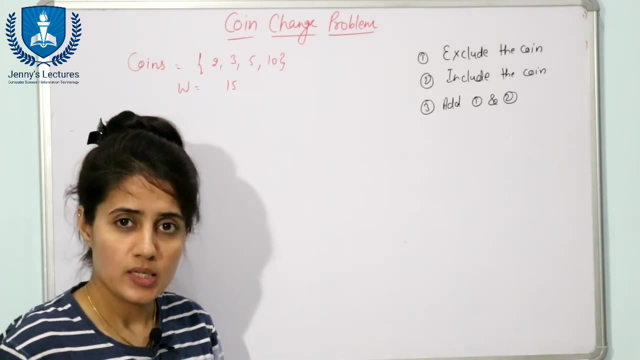 amount using these coins, and the condition is you are given infinite supply of coins. fine, now, using dynamic programming. how to calculate this thing? see we will. we can use recursion also. but what is the drawback of using recursion that we have discussed in previous video? fine, because the time complexity would be exponential. two raised to power and and why so? because the sub problems are computed again and again. okay, so what is the time complexity? the time complexity would be exponential, two raised to power. and. and why so? because the sub problems are computed again and again. because the sub problems are computed again and again. 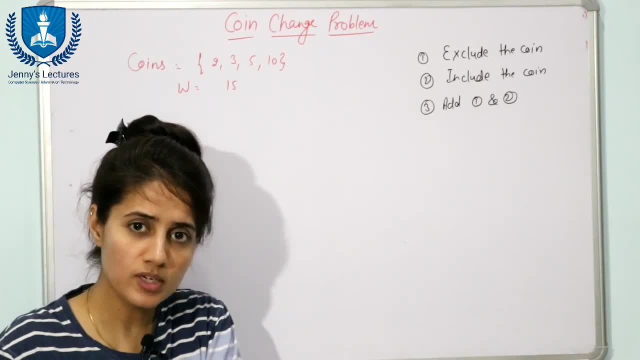 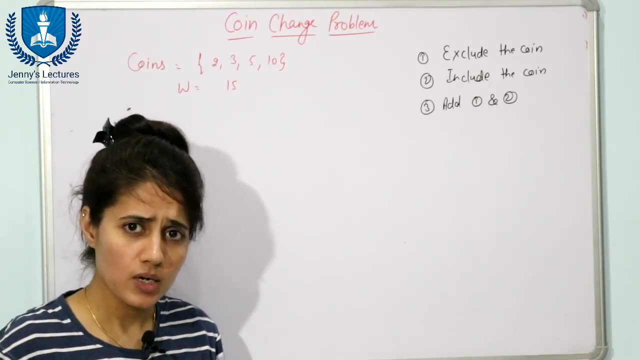 We are not going to store the result, but if we use dynamic programming, then we will store the intermediate result and we will use those results whenever the same sub problem comes in future. That is why dynamic programming will take less time, Okay, And number of computations will be less obviously. 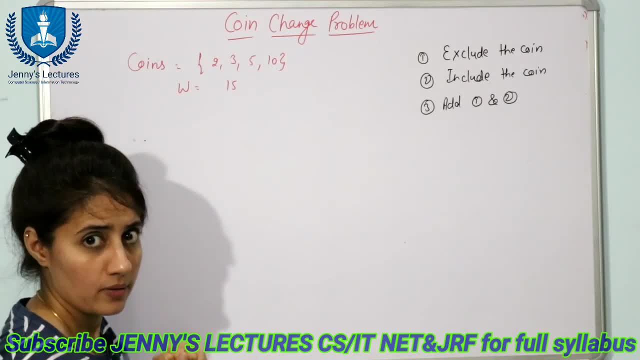 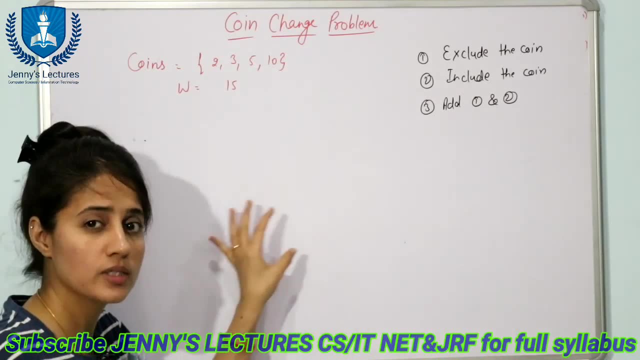 Now see how to solve this problem using dynamic programming. We are going to generate a table. Why so? Because we are going to store the results in that table so that we can easily use those results, those intermediate results. Fine, So this way, we are going to write the coins, the denomination of coins, 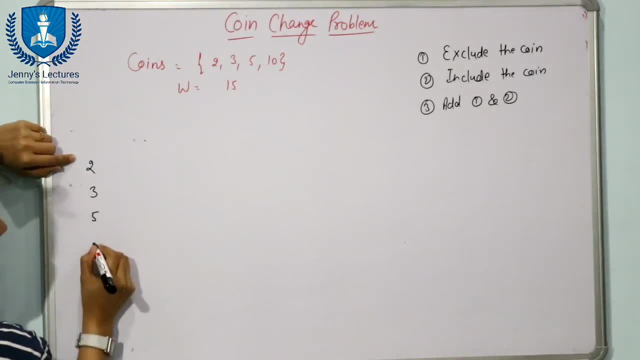 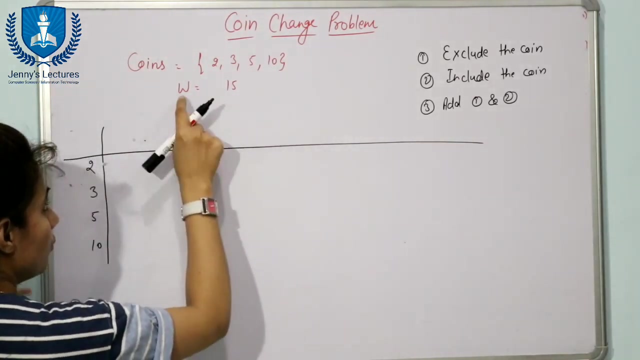 We are having 2,, 3, 5 and 10.. Fine, Generally we write these denomination in that ascending order. Okay, And this way, in this side we are going to use this amount, but we will not write 15. 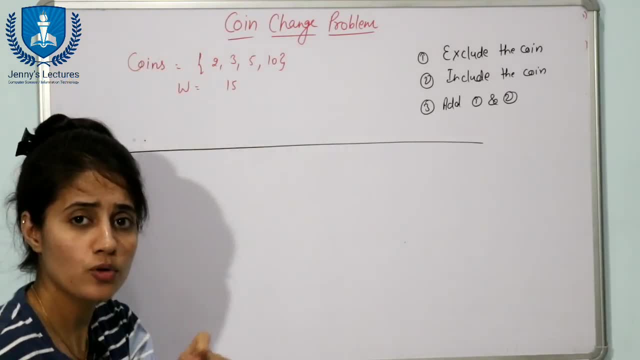 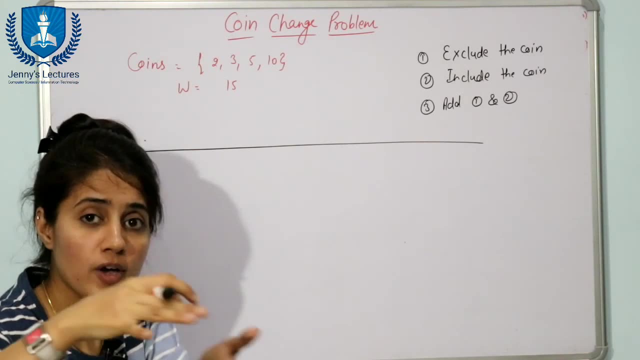 here because we are going to divide this problem. In dynamic programming we are We are going to divide the complex problem into sub problems. So we are going to divide this sum into smaller sums. So we are going to start from zero and till 15, we will write here: 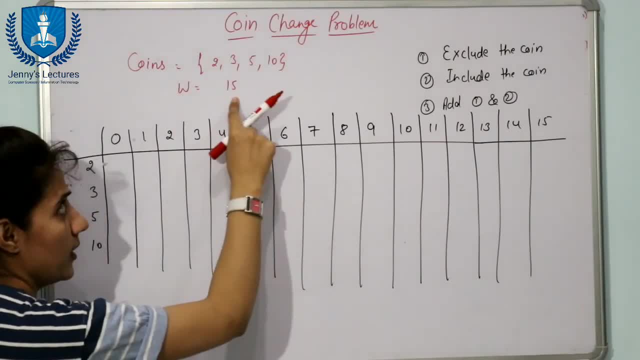 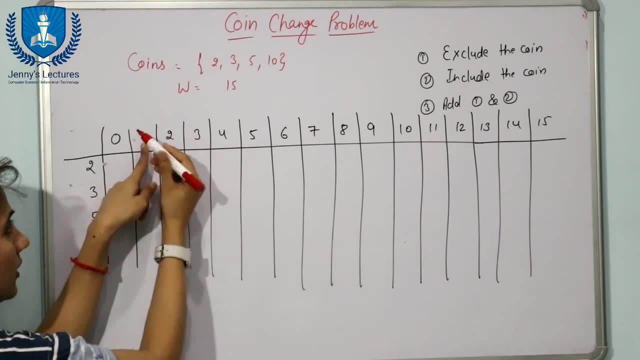 Okay, Zero, then one. Now we have divided this complex problem into simpler sub problems, like from zero to 15, you can take this one Suppose at time when we are supposed to make the change of this amount, one using these: 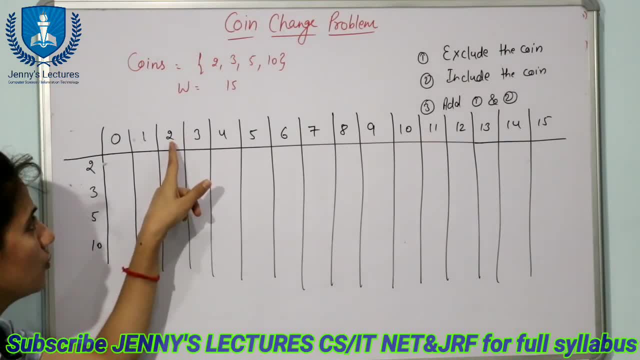 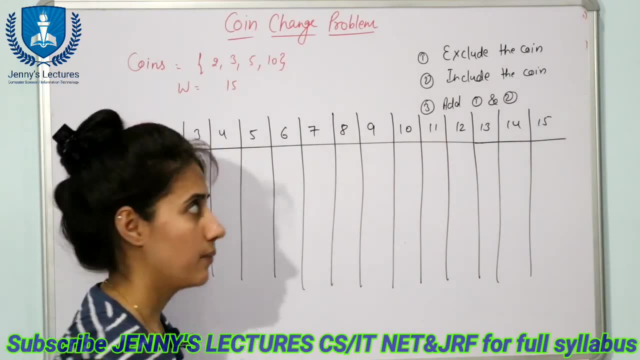 coins. At some point We are going to make a change for this amount using these number of coins, And ultimately we will reach to solution of the complex problem. Okay, So here, three simple steps are there. First is exclude the coin. 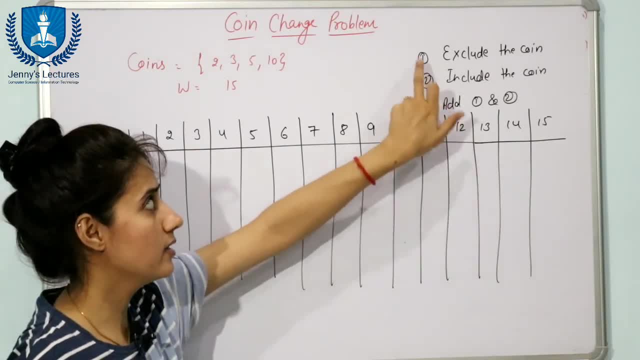 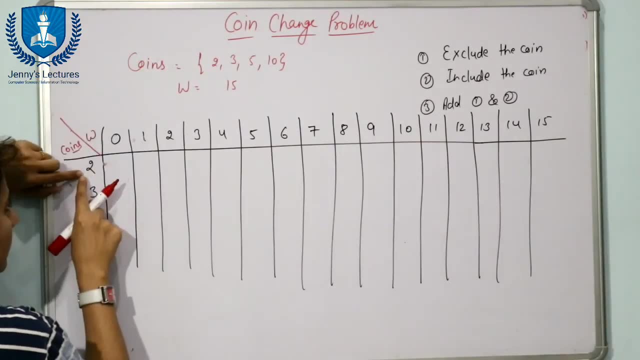 Next is include that new coin, or third is add this first and second. Now how to use these steps. I'll show you in this case at starting. suppose we are, we are at I value. Suppose this side is we are taking I value. 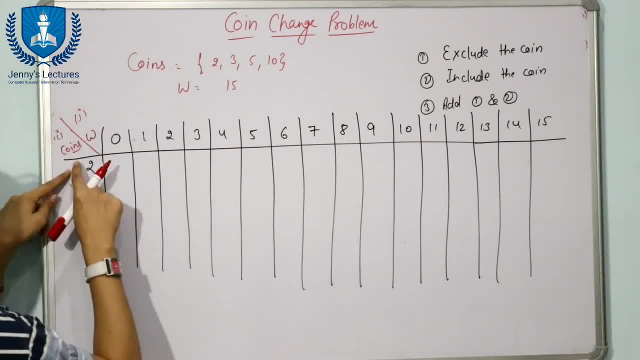 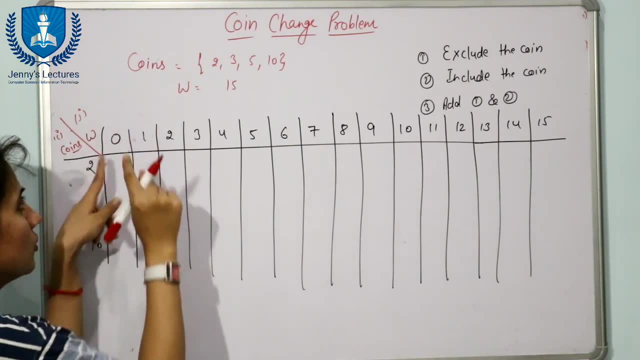 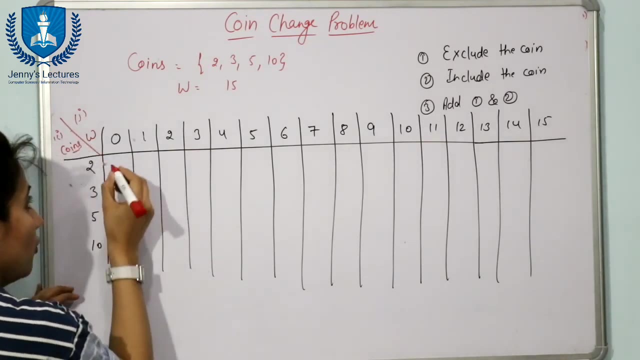 This side, we are taking J value. Okay, Now, when we have only coins of denomination two and the sum is zero, you have to make this sum. Is there any way? Yes, there is a way, one way, and which is that way? 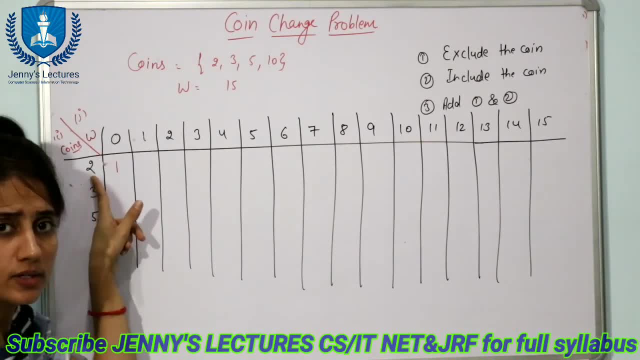 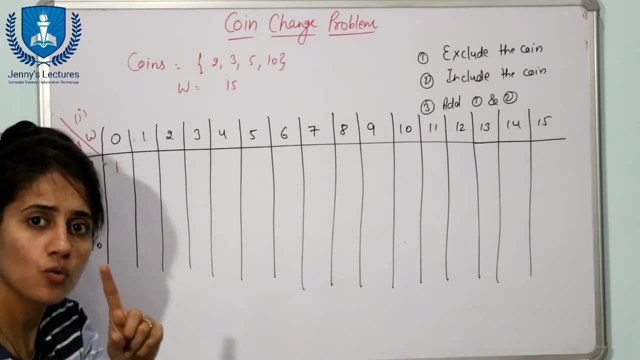 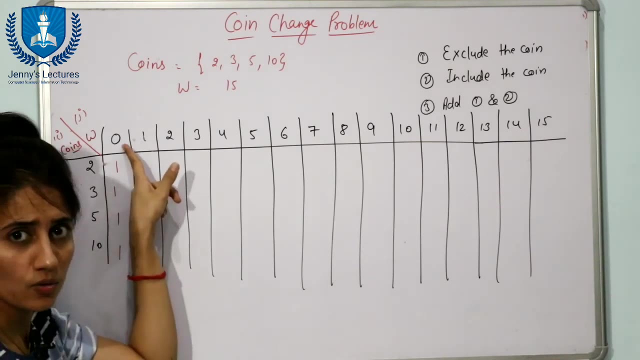 Because if you do not choose this coin, this coin of this denomination, then obviously you will make some of zero. na don't use any coin, So there is one way. So in this, In this problem, we always write one one, one below this zero, because if we do not, 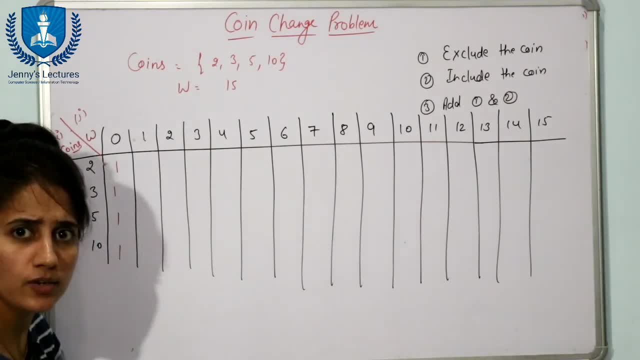 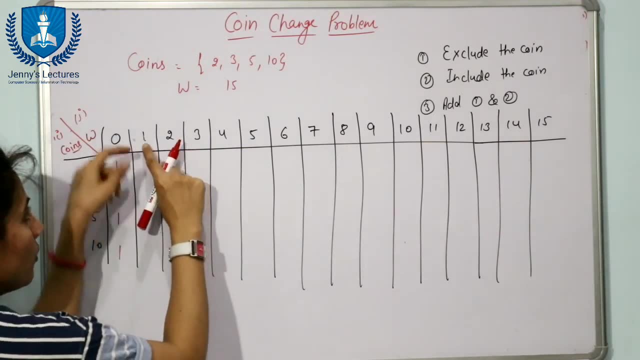 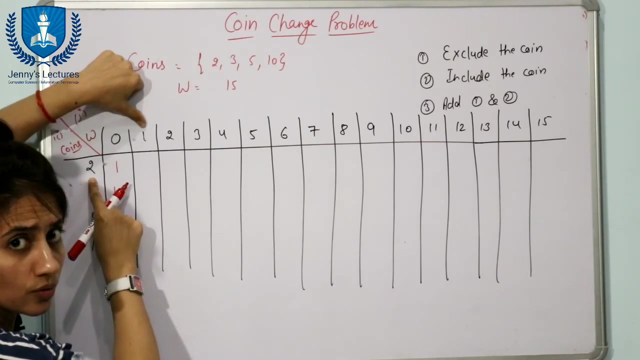 use. if we do not choose any coins, then obviously we are going to make a sum of zero. That is why we are taking here one. Now come to this point. Now the sum is one. Can you make this sum using a coin of denomination two? 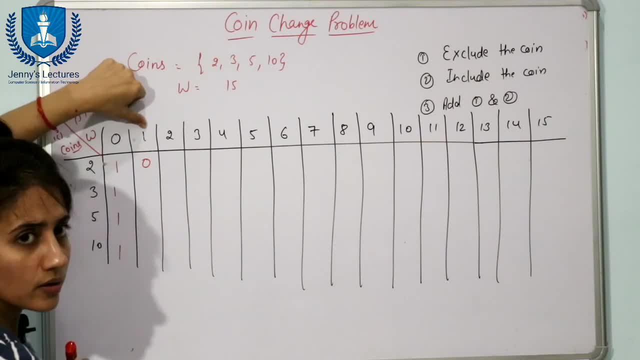 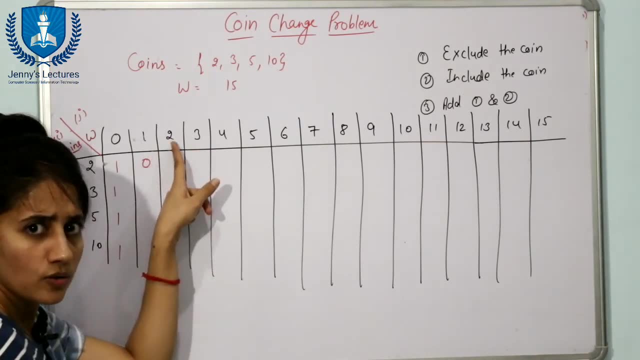 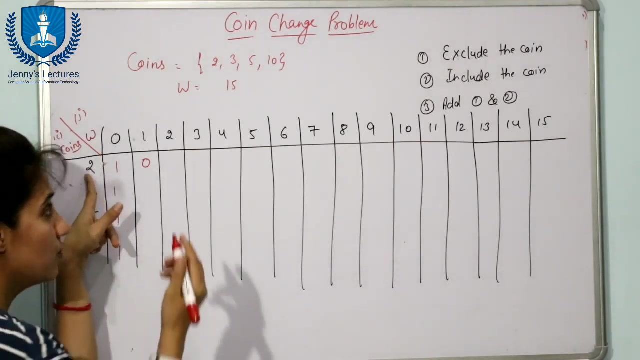 You can't Fine. So here you will write what: Zero. Okay, Now, next is two. Now see, sum is two and you have to make this sum using a coin of denomination two. Is there a way? Yes, we can do. 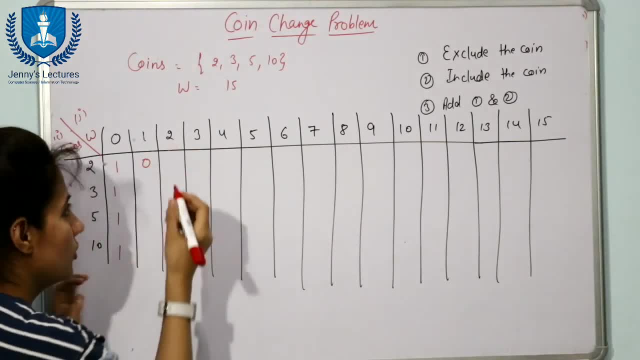 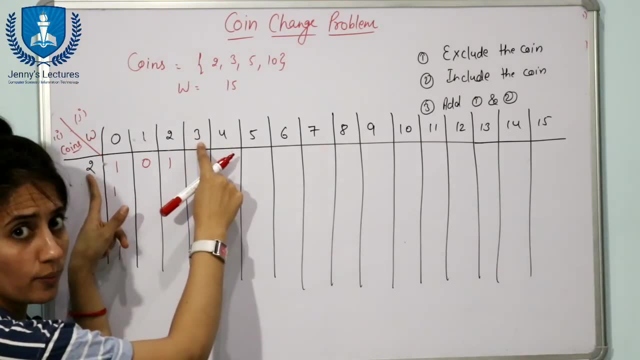 If we choose one, two rupee coin, then obviously we can take sum of two na. So that is why we have one way: Can you make a sum of three using coin of denomination two? If you choose one, two rupee coin, then you cannot make. 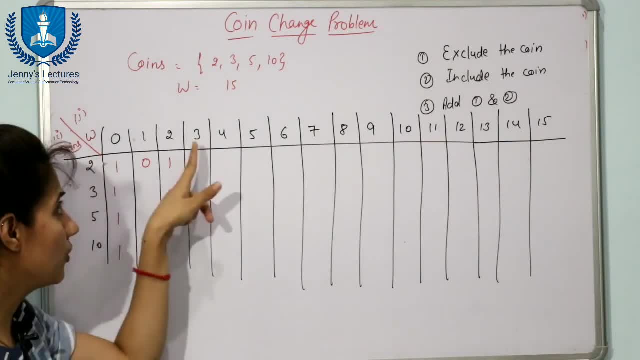 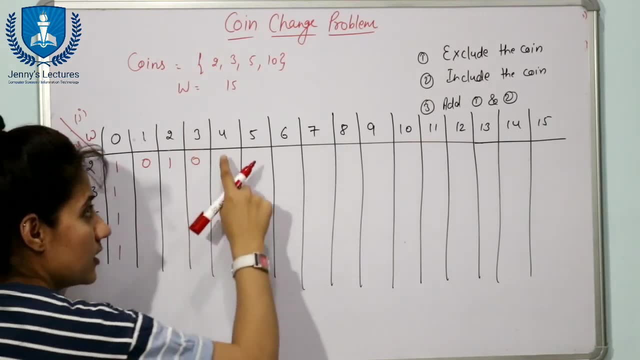 If you choose two, two rupee coin, then also sum is four. You cannot get three in any case. So there is no way. okay, Simply you will write some. you can make this four. Yes, we can make Only one way we have. 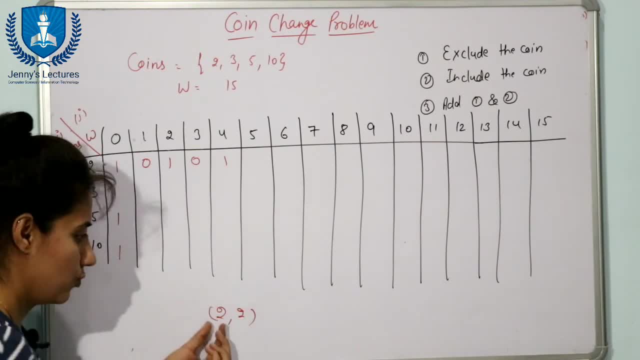 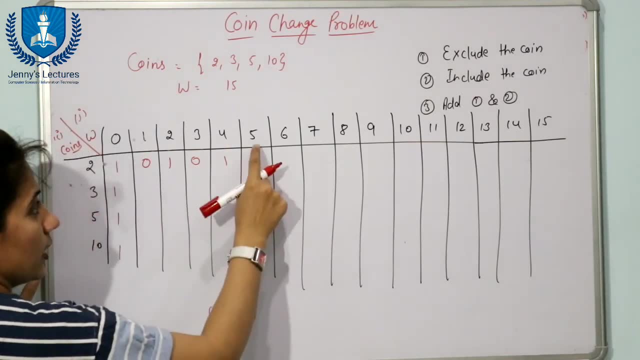 Which way is this? Two and two, Two, two rupee coin you choose and you will make a sum of four. So that is why we are, we are having only one way. Can you make this sum five? No, Can you make this? 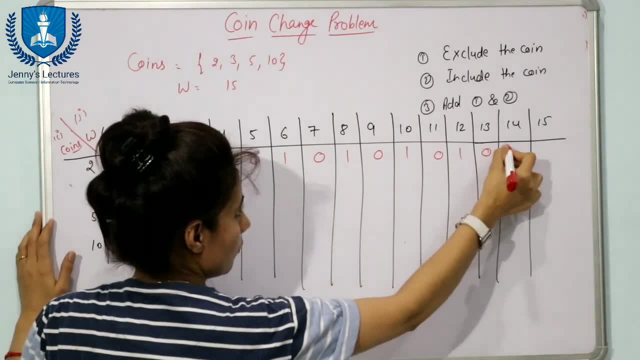 Yes, This, no This, yes, Zero one, zero one, zero one and zero Fine. Now i value is increased. We are having now coins of denomination two and three. Now the new coin is this: three Fine. Now, here we are using this rule, but simple rule is what you can say. 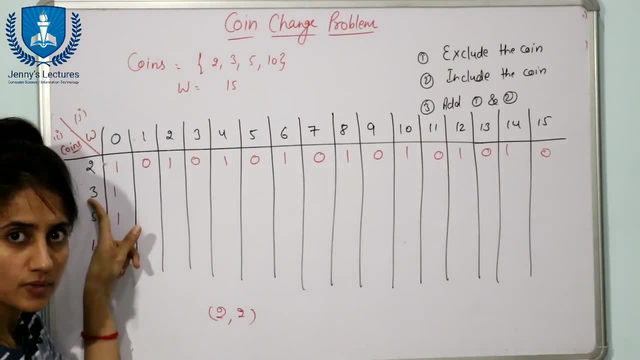 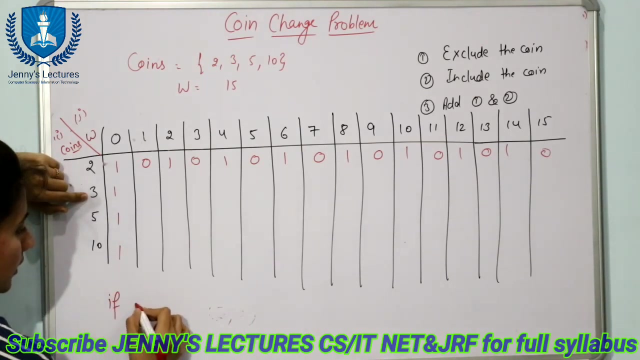 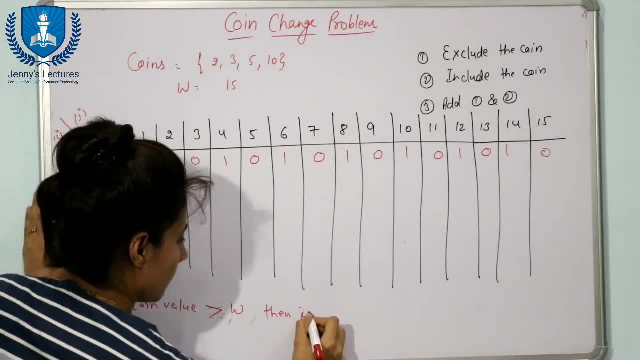 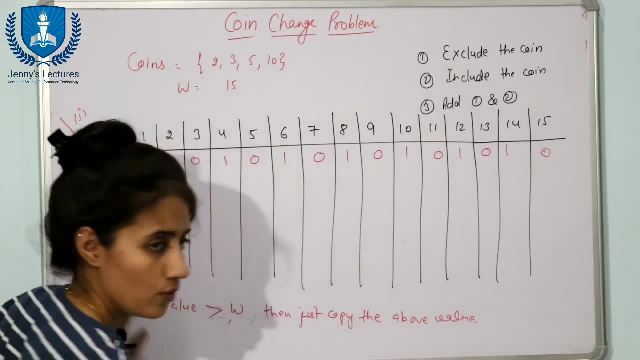 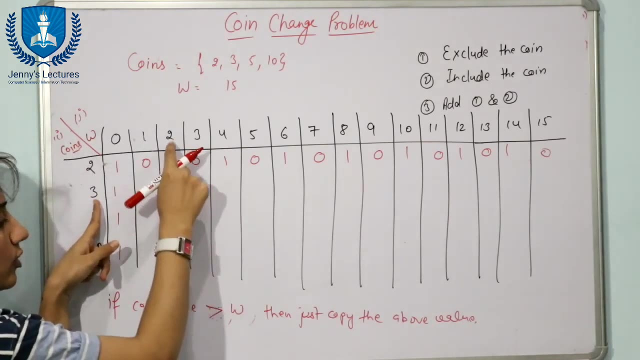 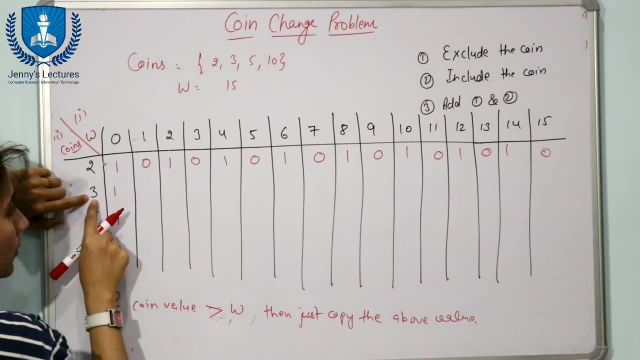 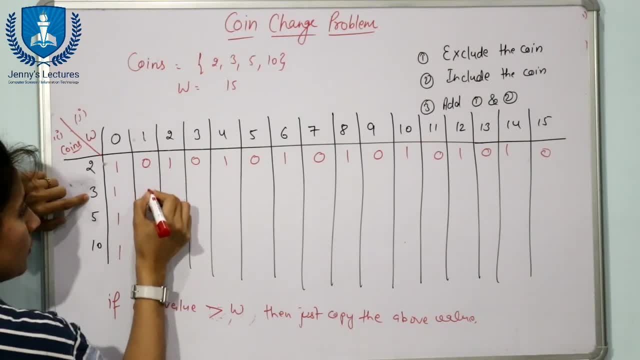 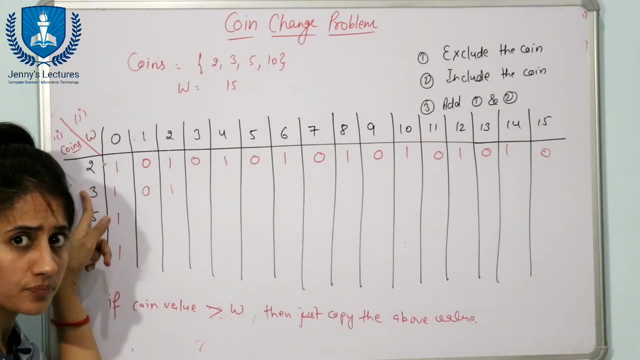 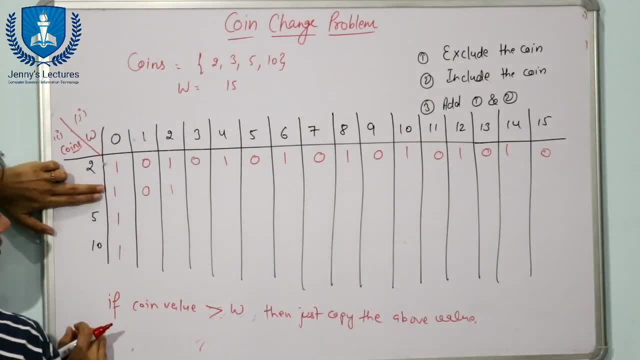 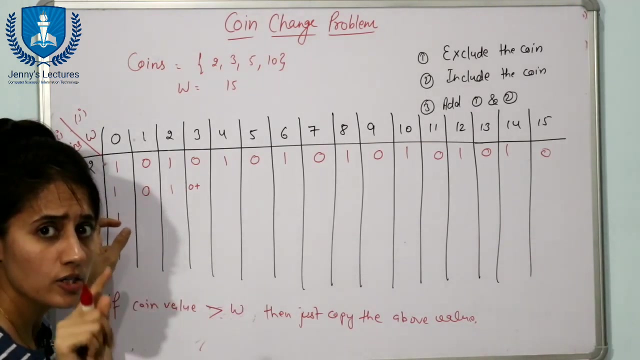 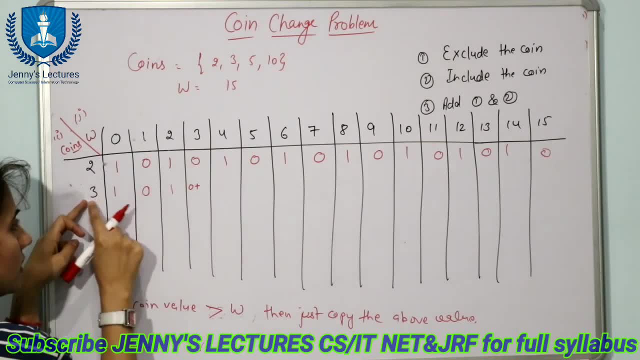 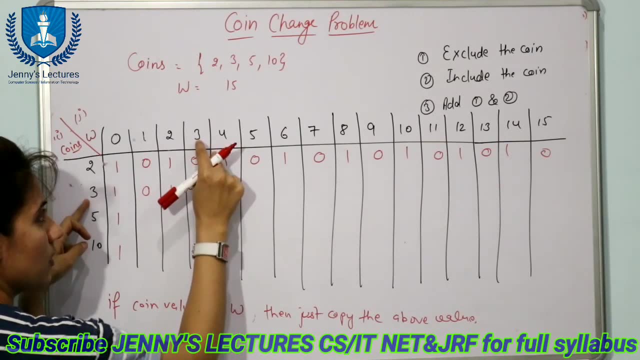 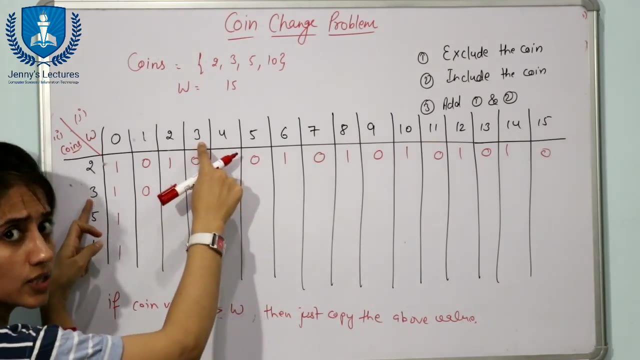 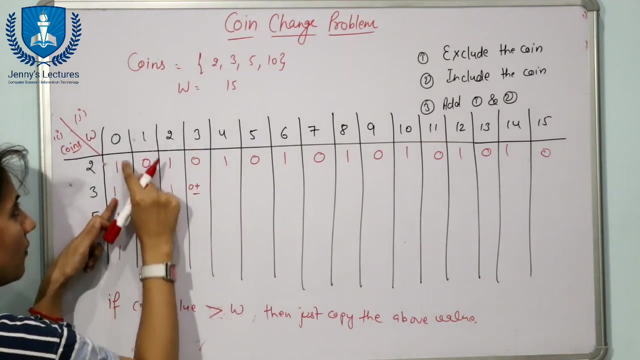 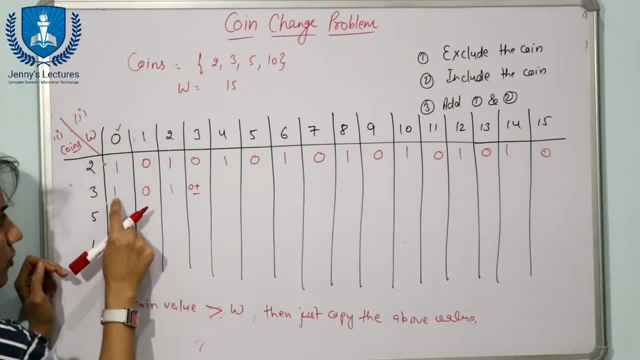 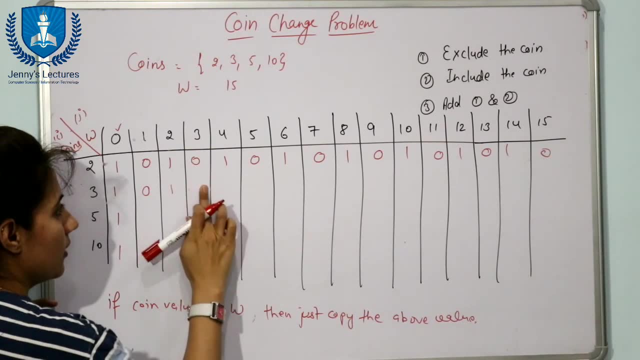 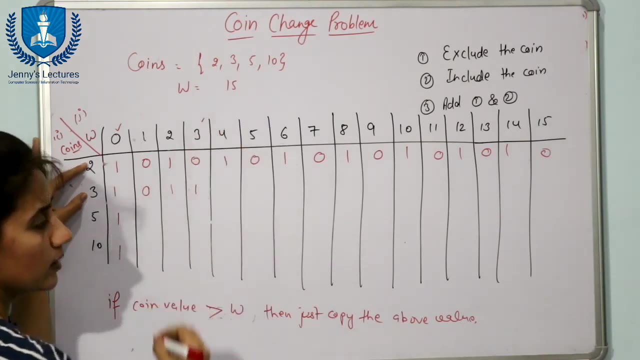 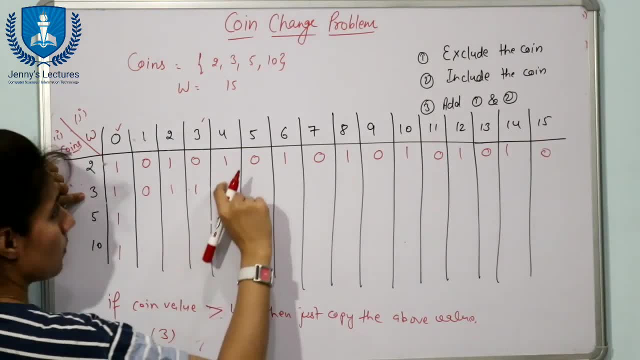 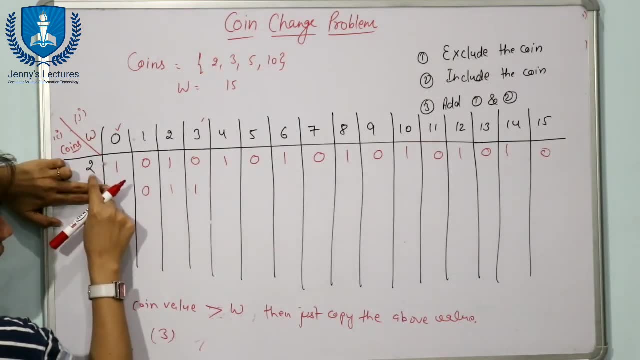 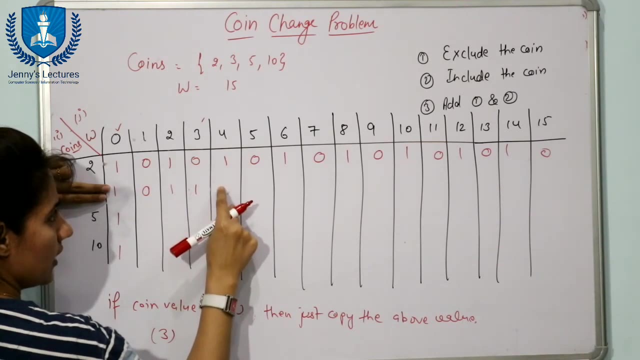 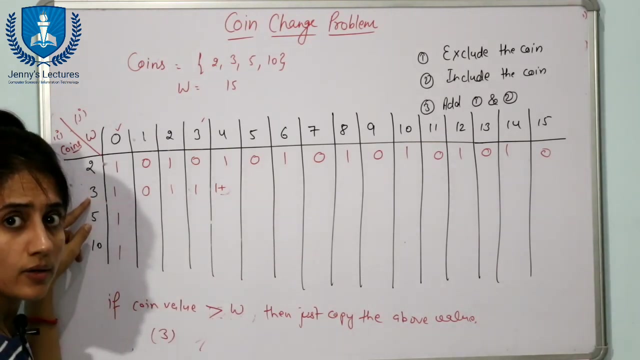 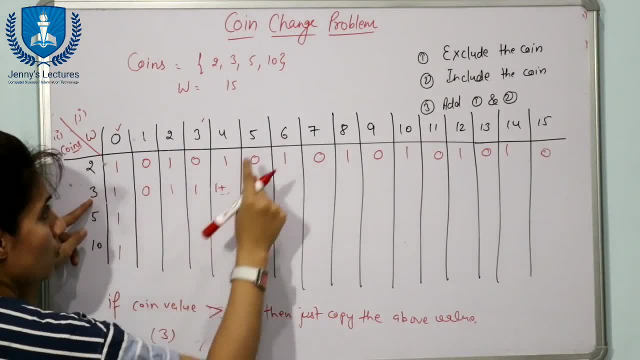 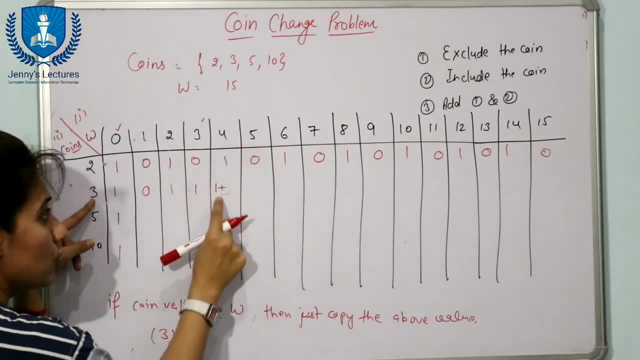 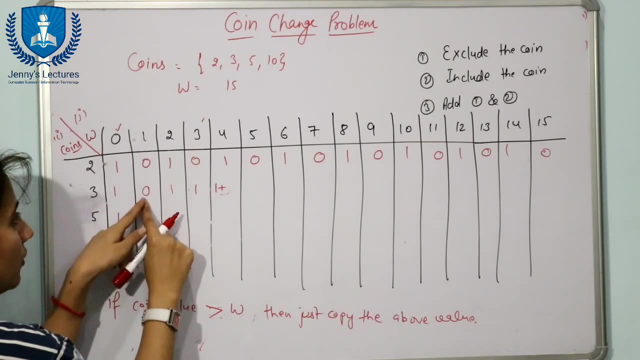 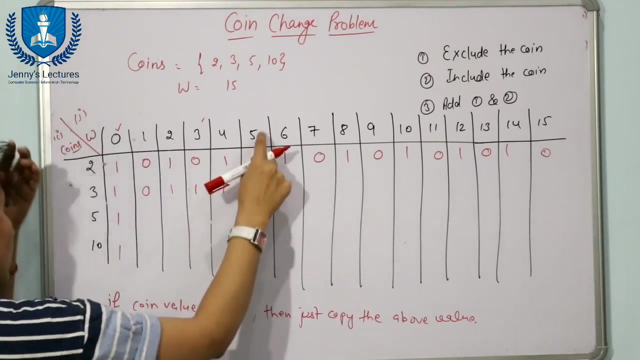 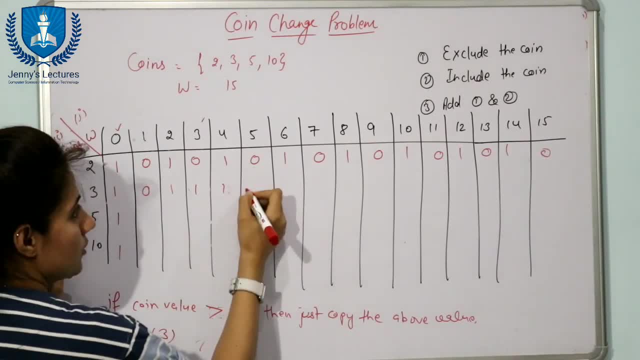 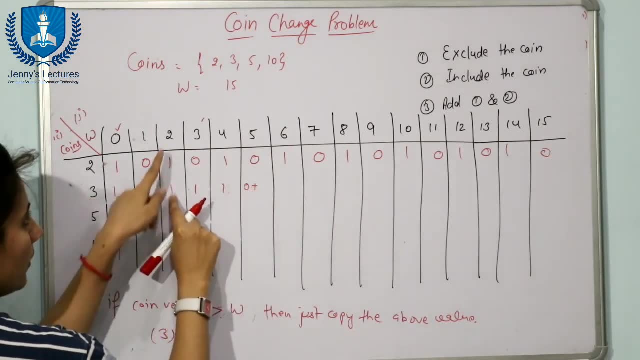 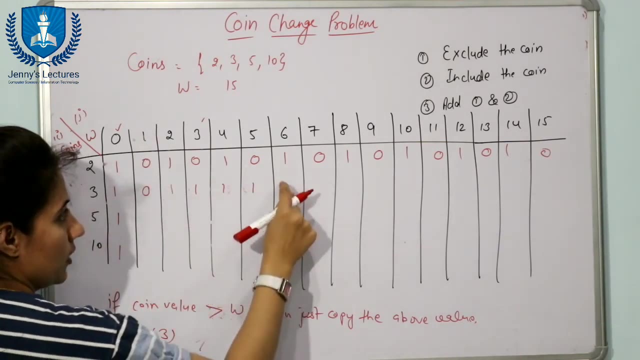 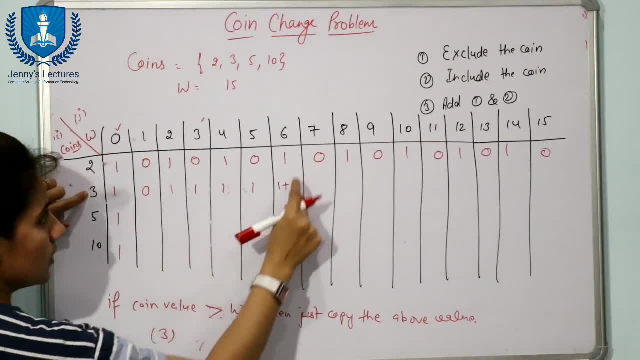 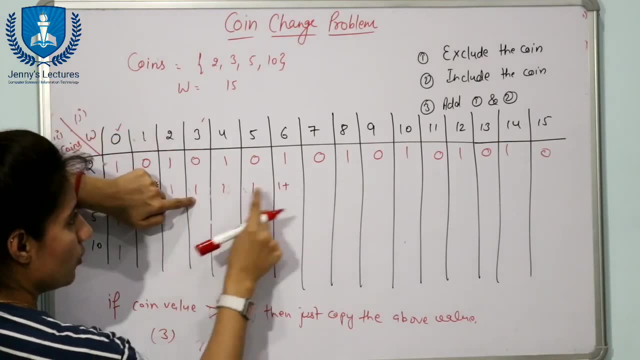 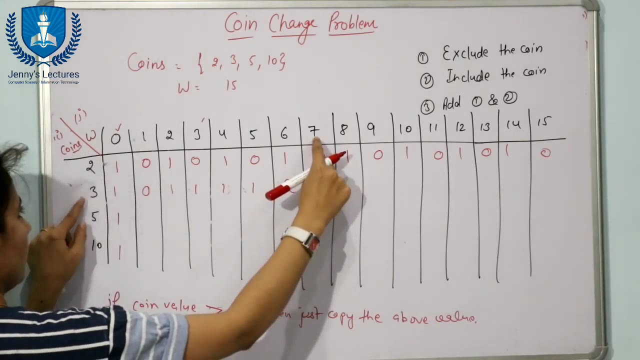 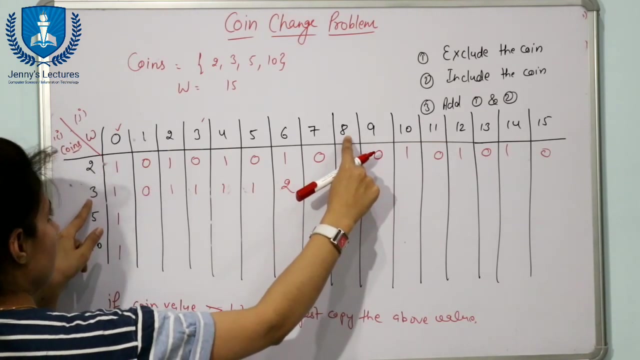 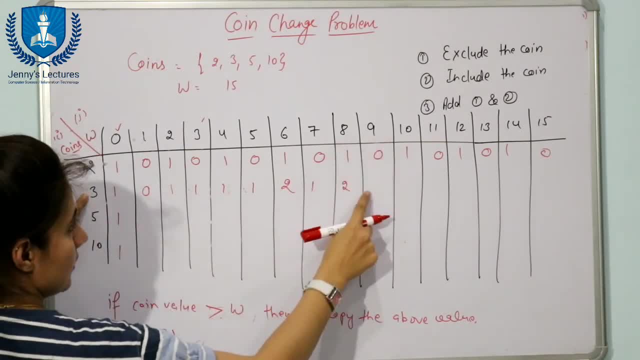 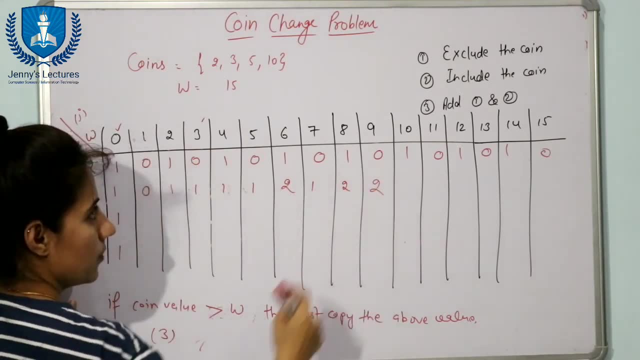 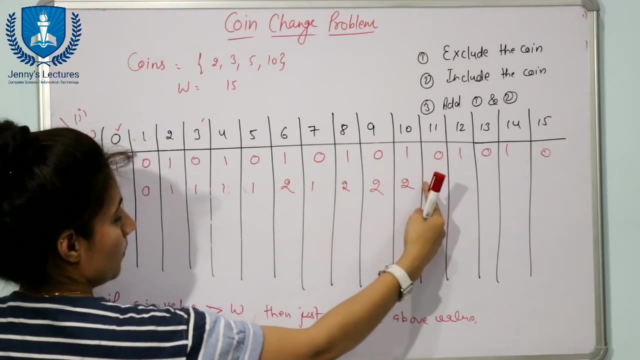 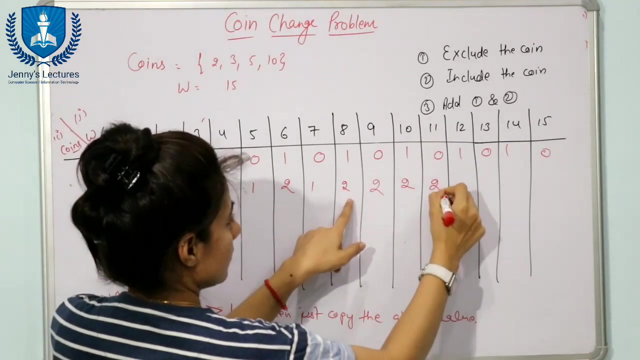 0 plus 9 minus 3 is 6 in this row. go to the column having sum 6: 0 plus 2 is 2 here. 1 plus 10 minus 3 is 7. 1, 1 plus 1 is 2 here. 0 plus 11 minus 3, that is, we have 8: 2 plus 0, that is 2. 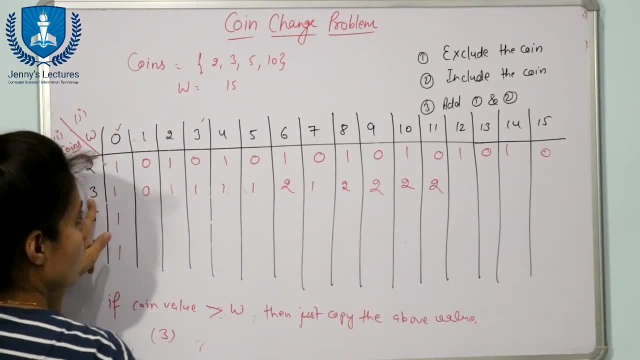 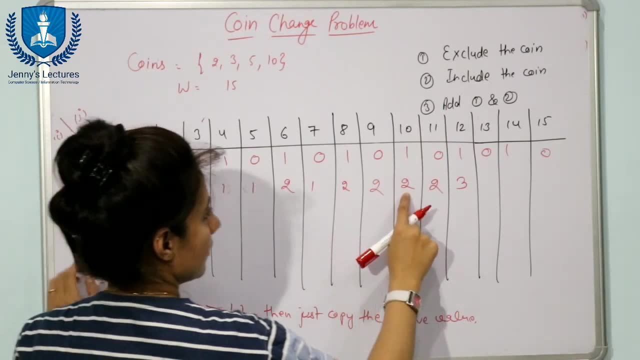 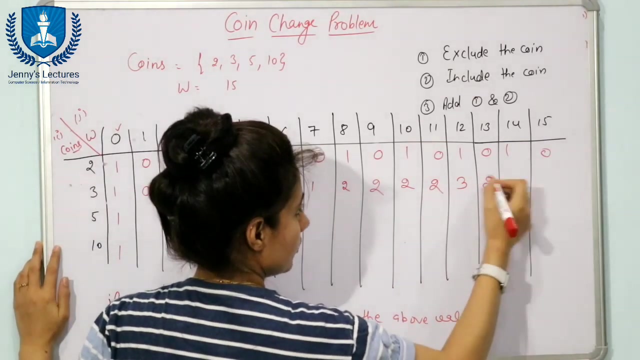 1 plus 12 minus 3, we have what? 9. so 2 plus 1 is 3. 0 plus 13 minus 3 is 10. we have 2. 1 plus 14 minus 3 is 11: 11. This one is 1 plus 2 is 3.. 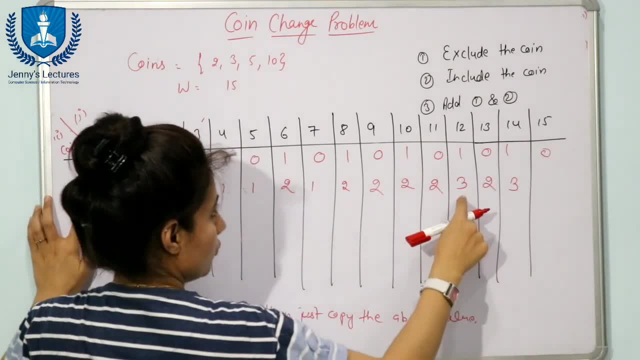 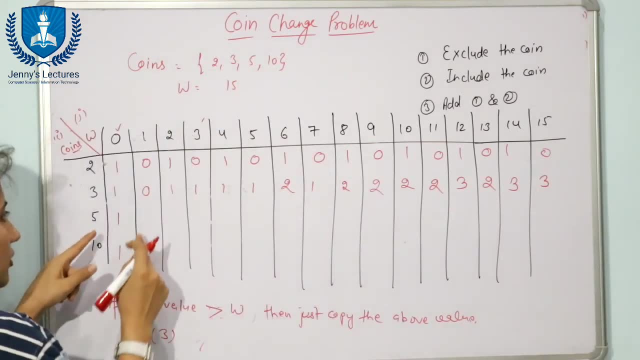 Here: 0 plus 15 minus 3 is, I guess, 12.. So here we will write: 3 plus 0, that is 3.. So let us take this case also. Now we are going to fill this cell. Now, here we have 5.. 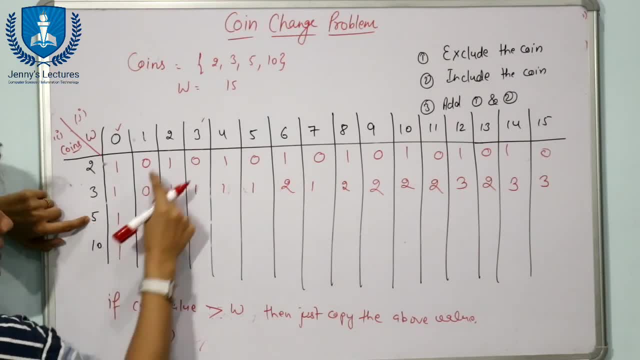 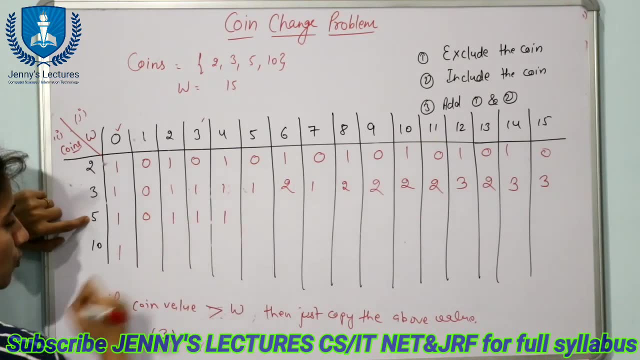 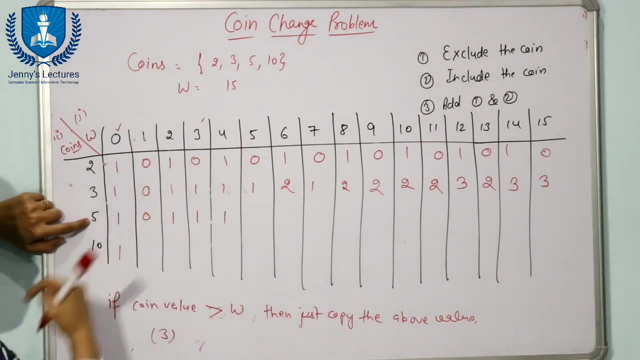 So this coin value, or you can say this row value, is greater than this 1.. So we will write just 0, here also 1, here also 1, here also 1.. Now, if you are here, we are having 5.. So from 0 to 4 you will write the same value which are in above cell. 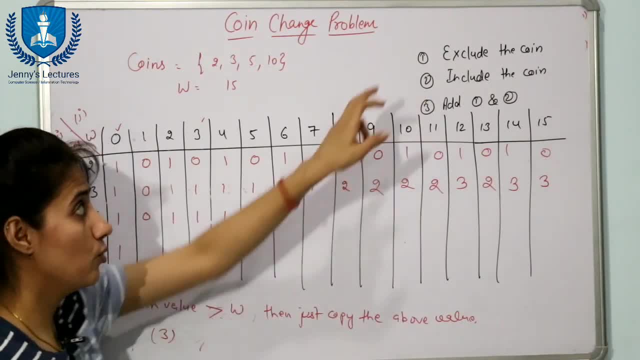 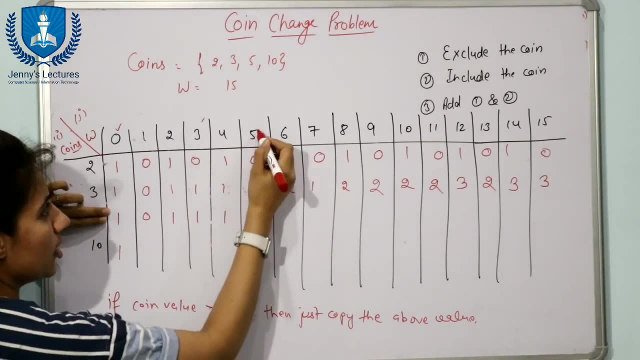 Now for 5. how to calculate? Simply include, simply follow these rules. Exclude this coin? fine. Now, if you are exclude this coin, then in how many ways you can make a total of 5 using only the coins 2 and 3? denomination of 2 and 3.. 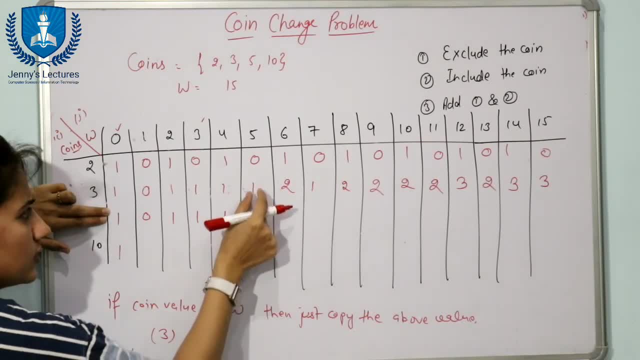 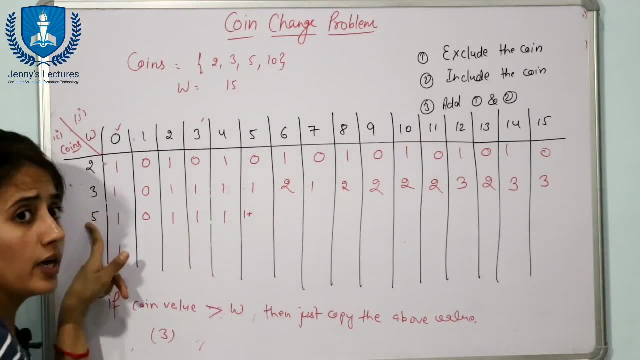 How many ways are there? One way is there: only Just copy the value of above cell. Just take the value of above cell Plus. if you include this coin, then how many ways? if you include this coin, then the funda is simply do 5.. 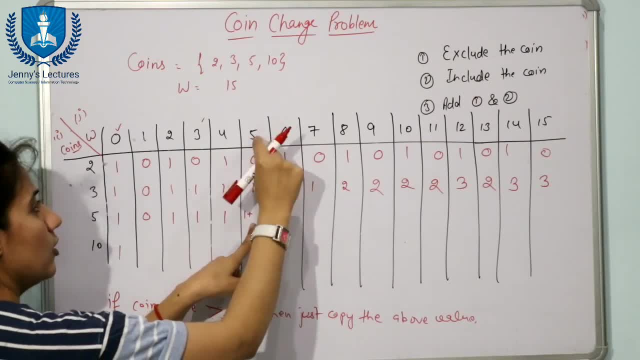 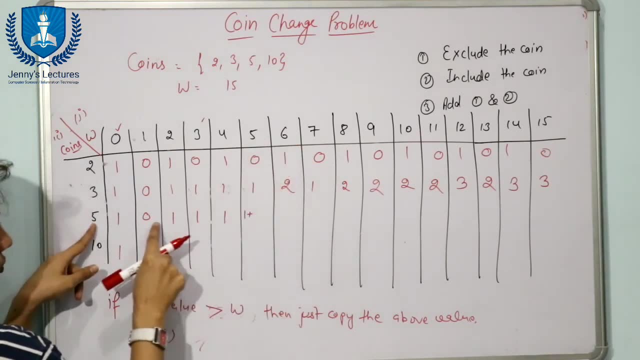 Just, we are going to calculate for this sum. So from that sum just minus the value of that denomination, 5 minus 5, that is 0.. So in the same row you will go to a column having some 0. here we have 1. 1 plus 1 is 2.. 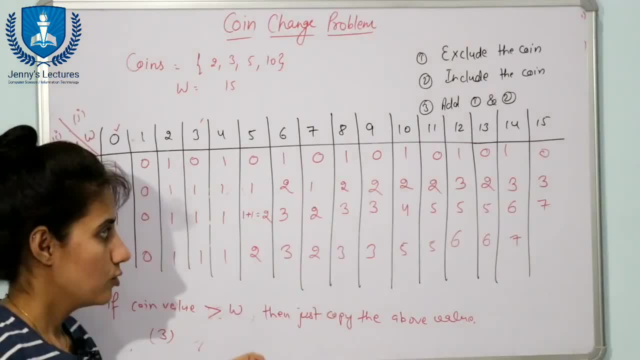 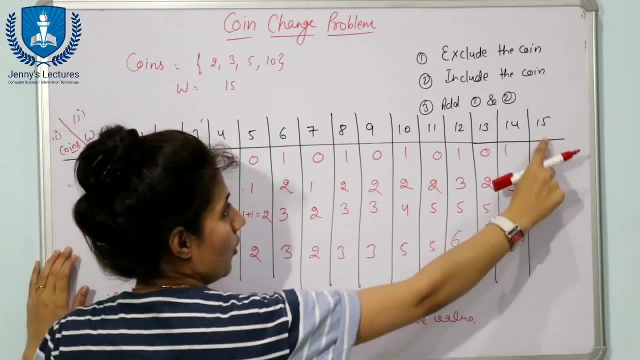 Okay, Now I hope you can fill this table like this. So, using that method, you just fill this table. Just check out for this. Just check out for this one. finally, See here, the amount is 15- and denominations: we are having coins of denomination 2, 3, 5 and 10.. 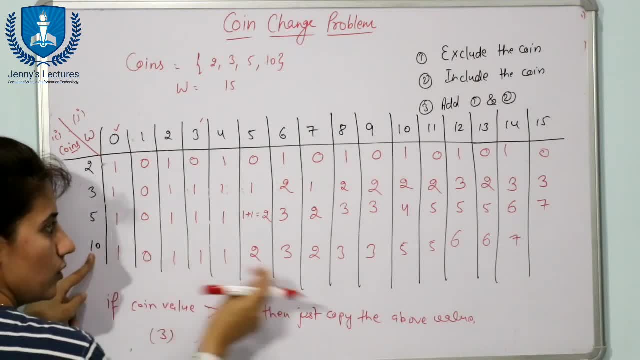 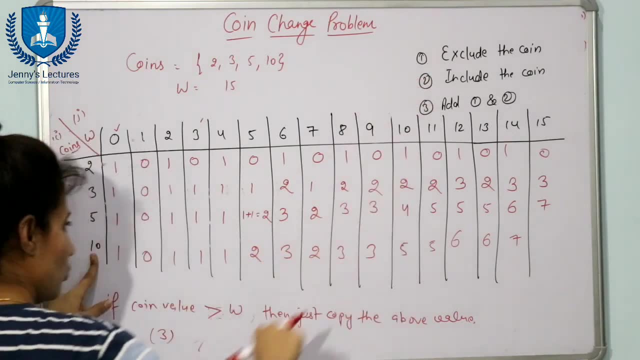 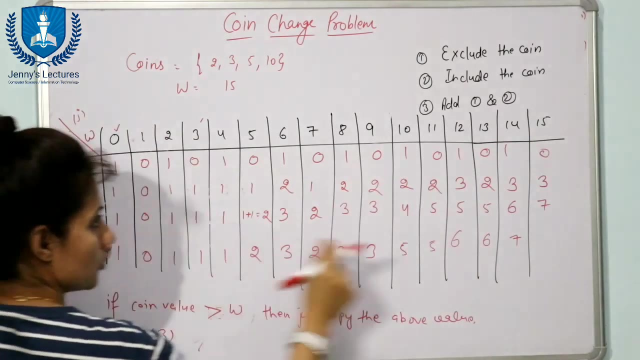 Now, this 15 is- you can say this- greater than this 10.. So we will not copy value from our cell. If this value is greater than that W value, then we will copy. Otherwise, you have to apply this rule. If you do not include this 10, if you exclude this 10, then how many? in how many ways you can get this total using these coins? 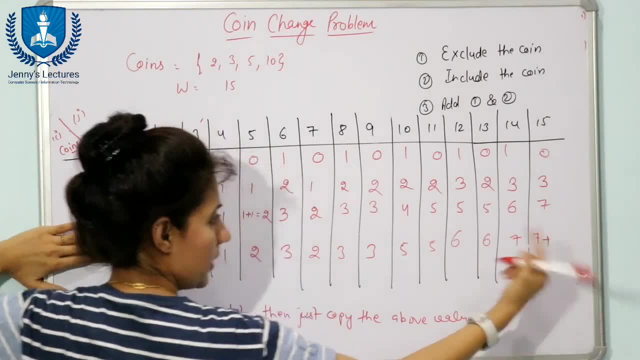 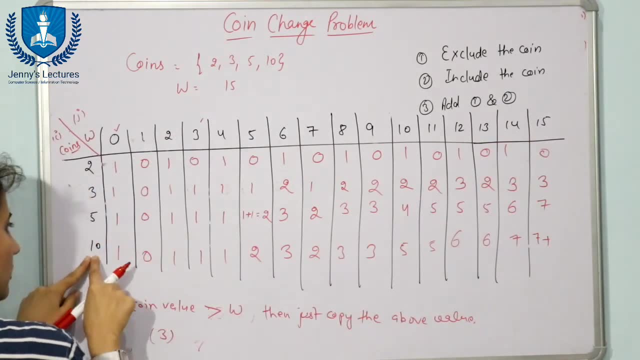 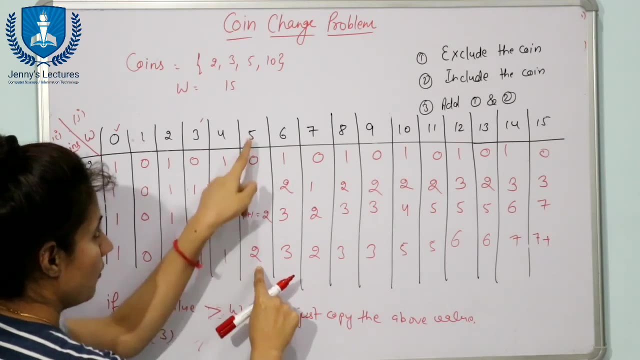 Obviously 7 ways. Just copy the value from above cell Plus. if you include this, then how many ways? Then the method is: just do this amount minus the coin coin value: 15 minus 10 is 5. And just in the same row, go to the column having value 5.. 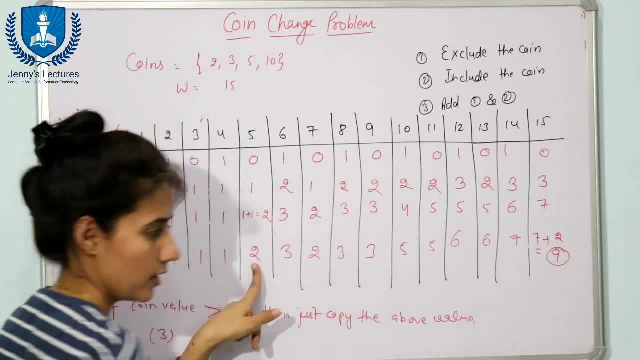 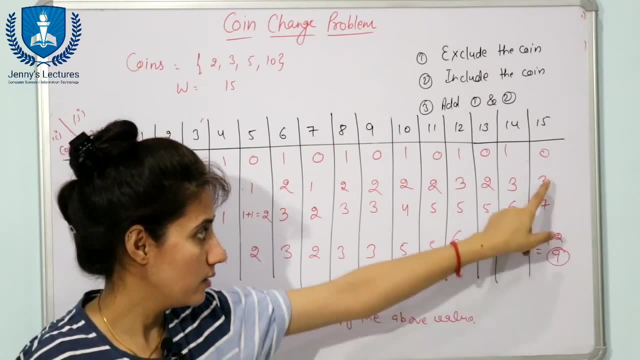 So here we have 2, 2, that is 9.. Okay, So how many ways are there? 9 ways. The answer would be always in the intersection of large Row and last column. So 9 ways are there in 9 number of ways. 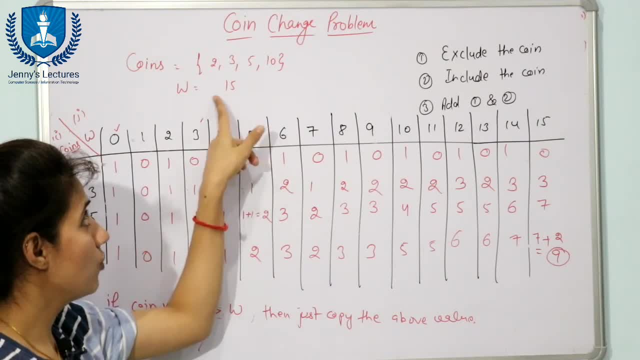 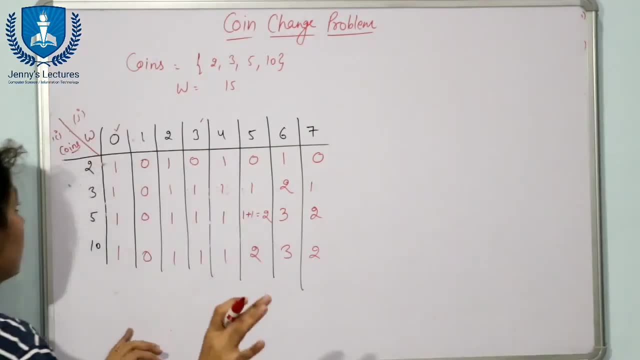 You can make a total of. you can make a change of this 15 using these coins. Now we are going to write the logic for this one. See, suppose I am taking a 2 day array, Okay, Where you are going to store the solution. 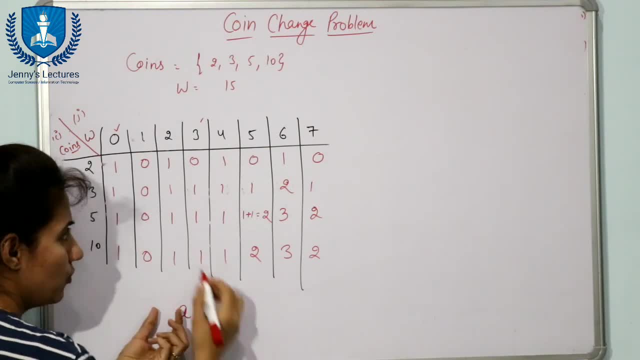 Suppose this cell is there, So I am taking name of, this is a and I and J. This cell is A of I value. is this one, This side, this side we are going to take I value. I value would be from 0, 1, 2, 3.. 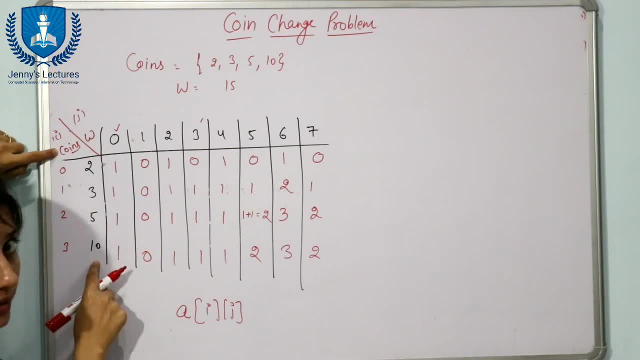 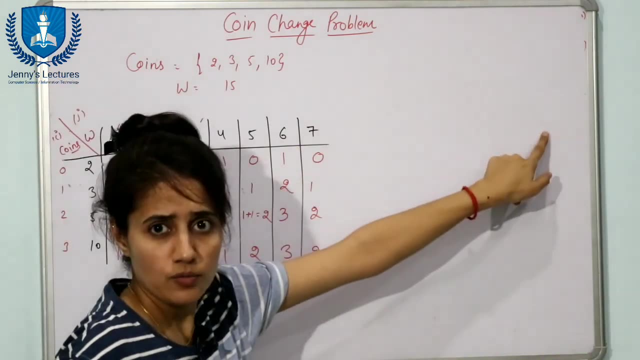 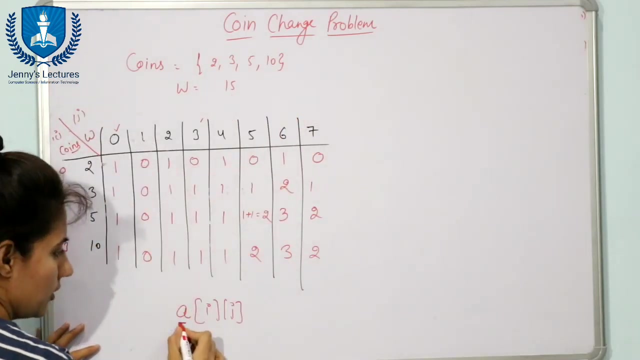 Coins. coins is the array 1 day array. we are taking, Okay, And here we are taking J, this J value from 0 to 0 to 15.. We have taken 0 to that amount. Okay, Now, and this, this array, I am going to take name A. 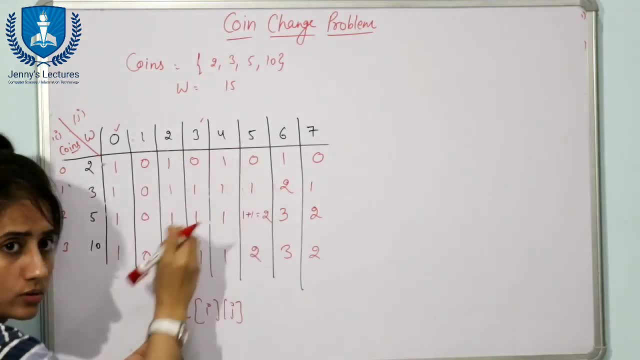 A 2 day array Where we are going to store this results, the intermediate results. Fine, Now you have to apply two for loops. What? what are those for loops? One is for this I and one is within this I, within this row. 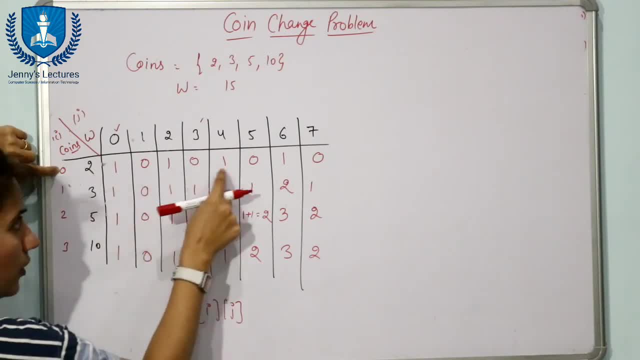 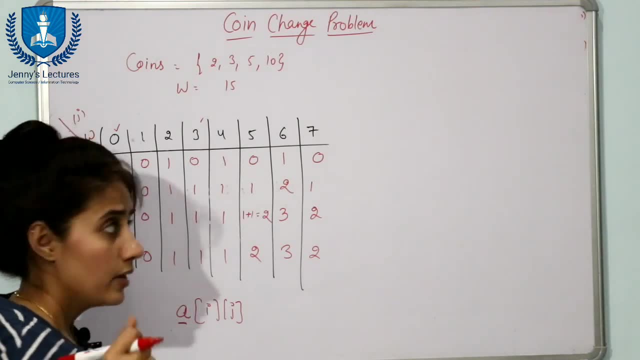 I is for row. within this row. We are going to check the values of columns now. So first of all for row, then within this row, for column, for two loops We are going to take first thing. What you have to do is Simply: we are, we are. we have just put 1: 1, 1 here. 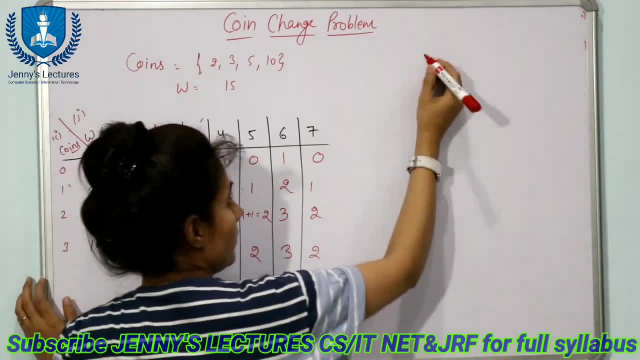 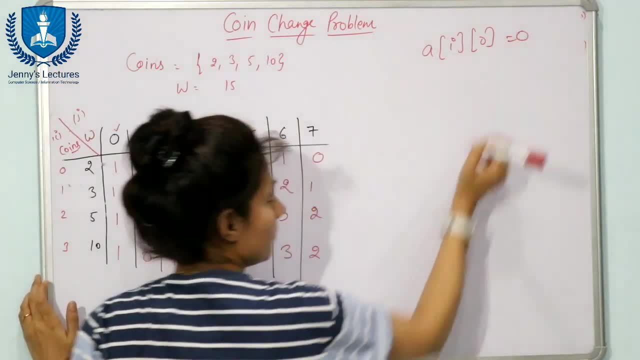 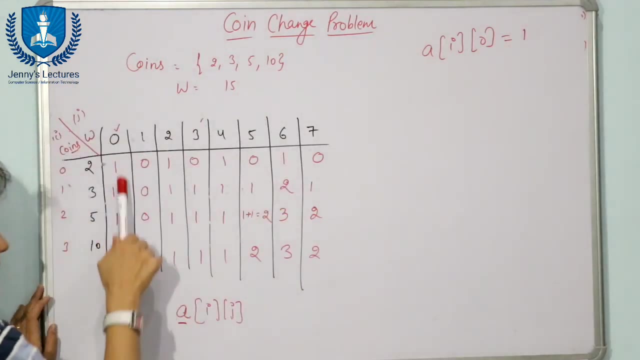 When the amount is 0. So maybe simply you can do A of I And column value is this 0. And simply put 0. Sorry, So I simply put 1.. At all the places and somewhere you find that They, they will start here from 0 denomination. 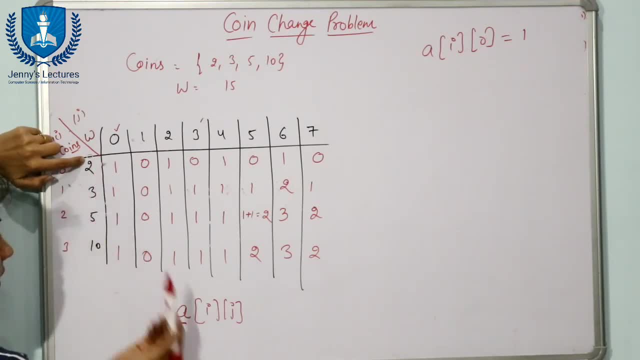 The 0, then 2, then 3, then 5 and 10.. So if 0 denomination you take, then what you will do Here only you will take one, otherwise 0, 0, 0, 0, 0, 0.. Because if you do not have any coin of any denomination, 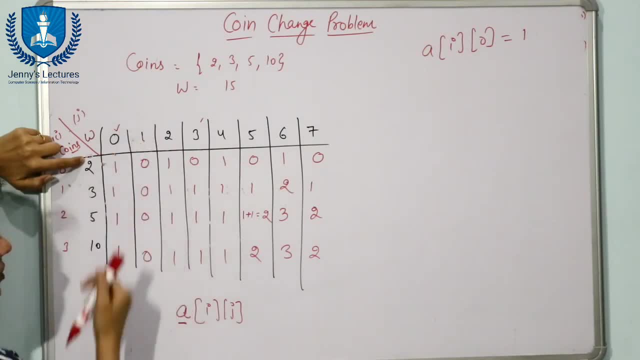 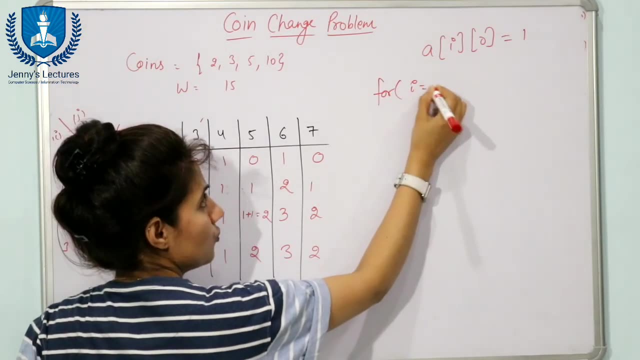 Obviously, then you cannot make the sum. You can only make a sum of 0 only. So now next thing is you have to apply the for loops. One for loop is for I. I is equal to from 0 to I less than equal to. 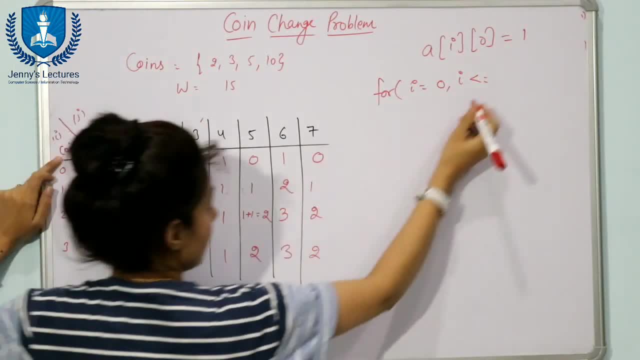 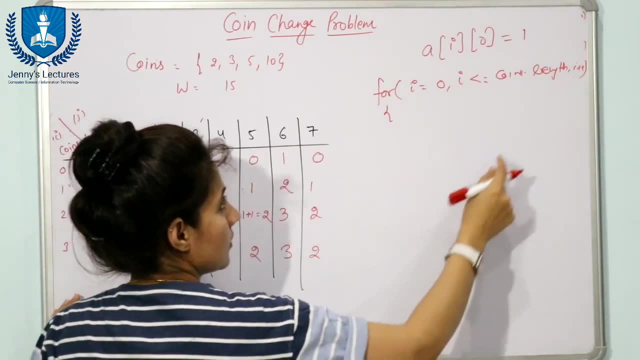 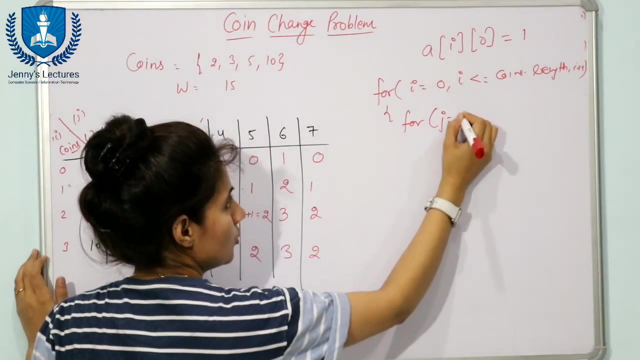 You can say that If you are taking this array, name is coins, Then you can say that coins dot Length and I plus. Then, within this loop, we are going to take a loop for J for these columns. So J is equal to 0.. 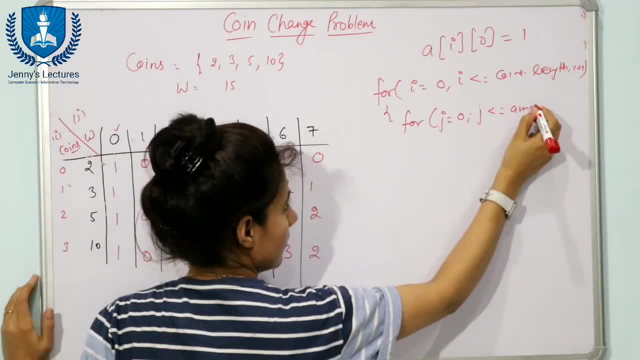 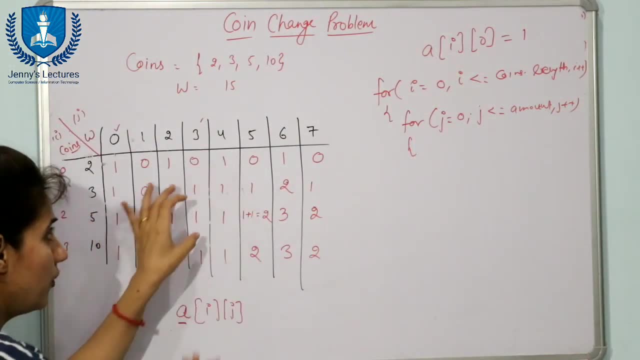 And J is less than equal to this amount, given amount, Amount and J plus Plus. Now you have to apply the logic. Have you filled these Sales? Okay? Simple rule is what If? If this Coin value, This row value, is: 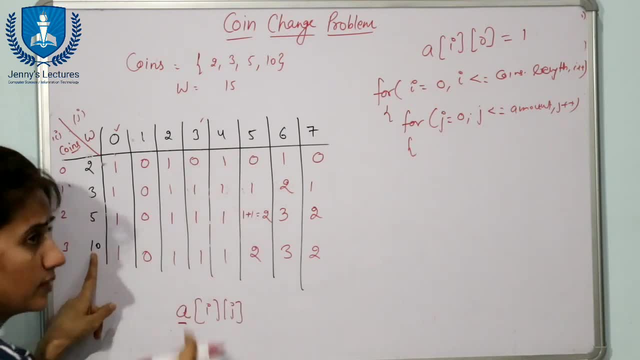 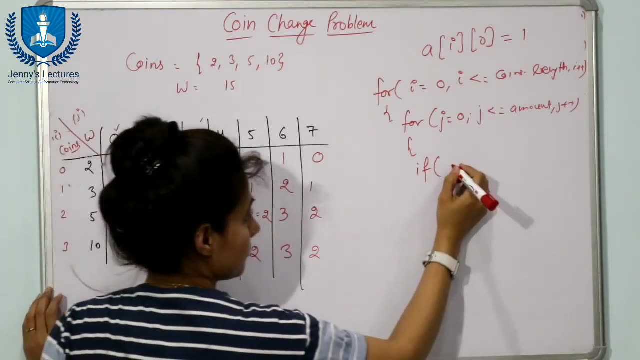 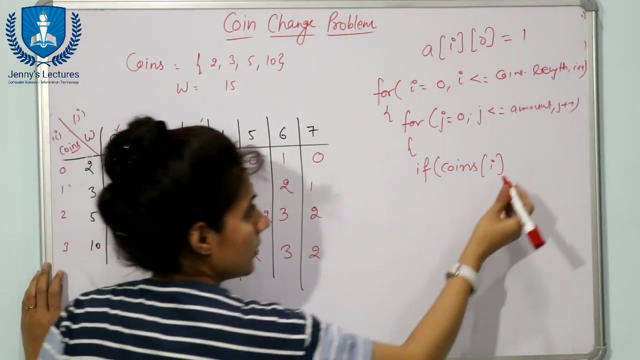 Less Row value is greater than this amount, Then simply copy the value from above cell. Fine, So just write down, Just check a condition: If Coins of I Is greater than J, Then what you will do, Simply. 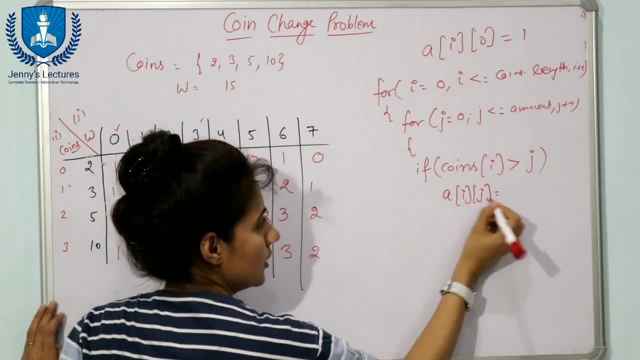 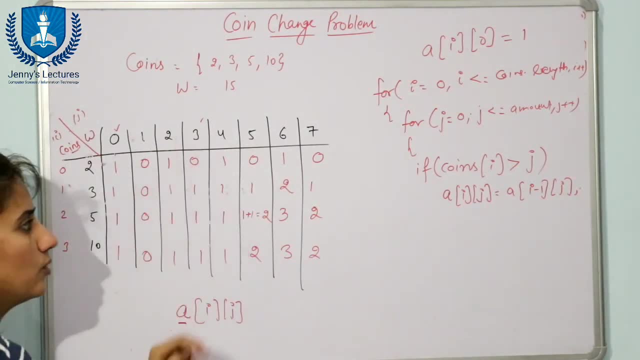 A of I of J is equal to A of I minus 1, and J I minus 1 means, From the upper row, Copy the same value. Else You will do what Else You have to apply the formula. 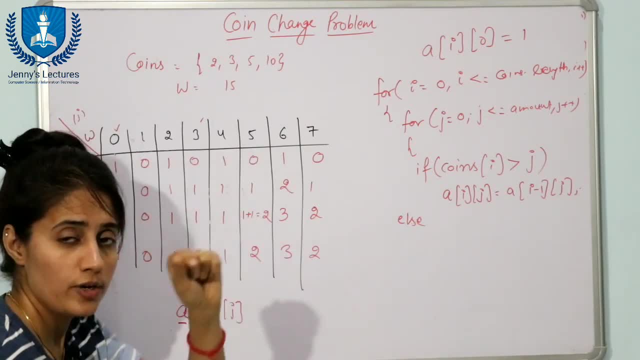 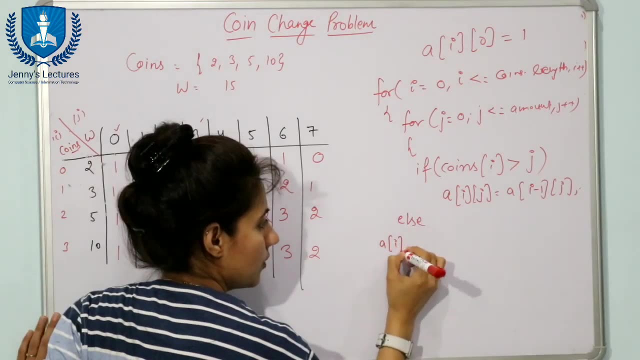 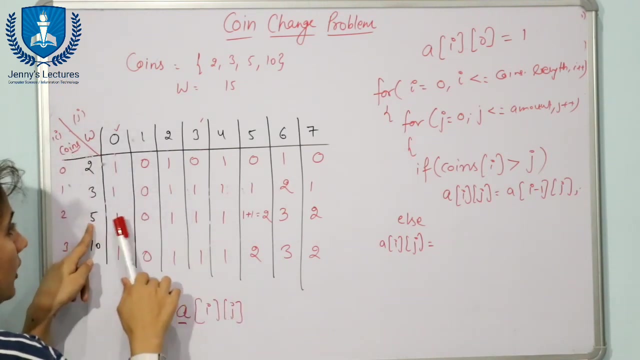 That exclude, Include And then add 1 and 2.. Fine, Now See Else A of I J Is equal to What We have done. Else See, Suppose This one was 5.. 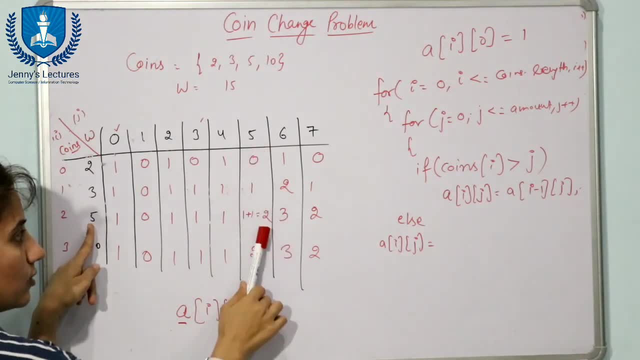 Till 0 to 4.. We have copied Same value Else What we have done This: This value Plus 5 minus 5.. Plus This value From 0th column, 1 plus 1.. 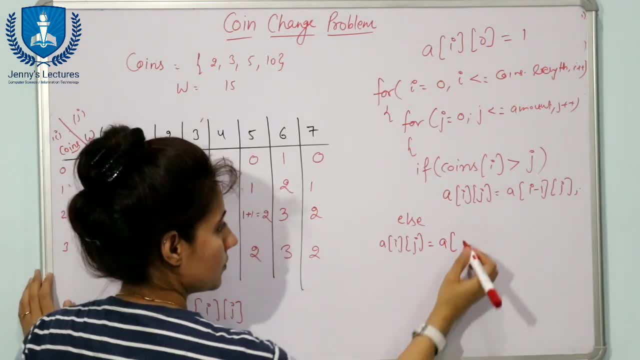 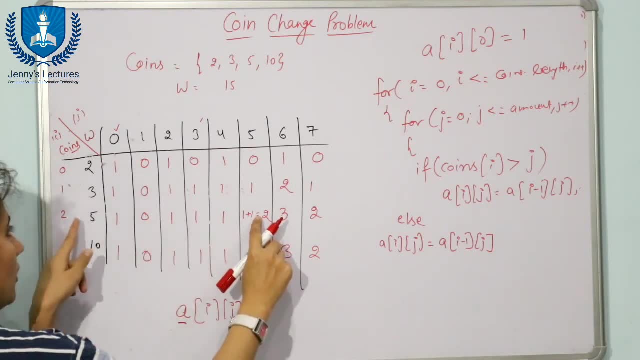 That is 2.. Now, What you have done is A of I minus 1. And J See A of I minus 1.. Is this one And J Is same row, So This: 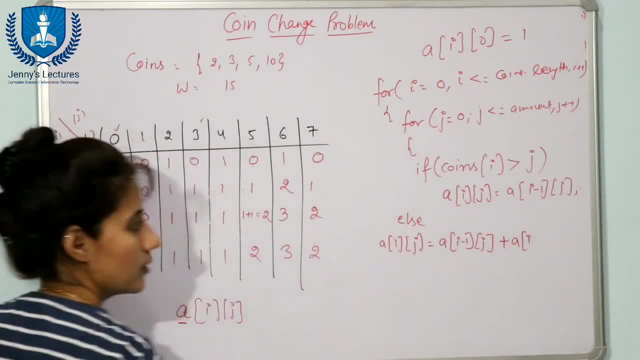 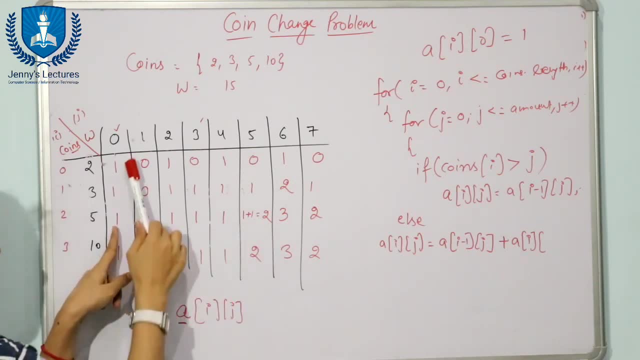 Value Plus Plus What we have done. A of Same row, I would be same, But We have changed The column Column value. What we have taken Column value is This one, So Column value is: 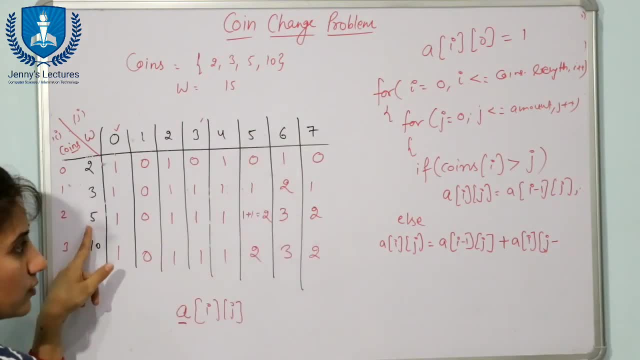 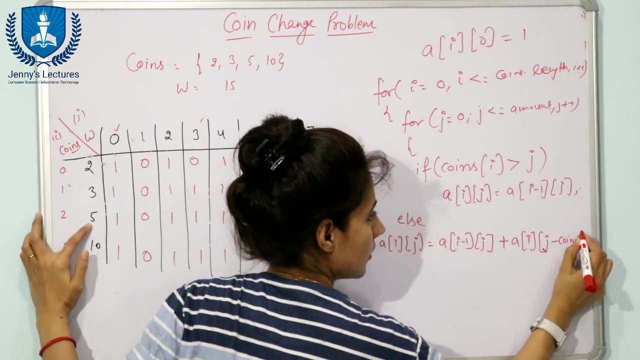 This J Minus What we have done, This 5 minus 5.. So Here J Value is This one, This 5.. Ok, Now From 5. We have Minus This value. 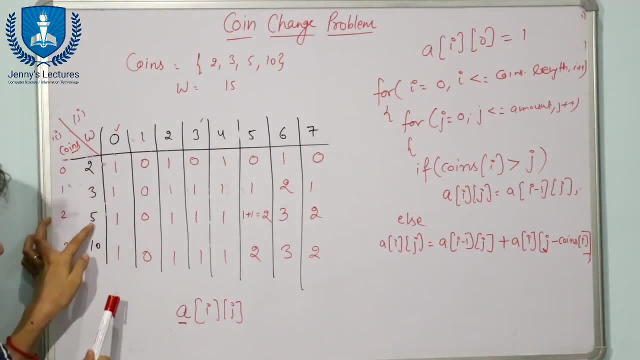 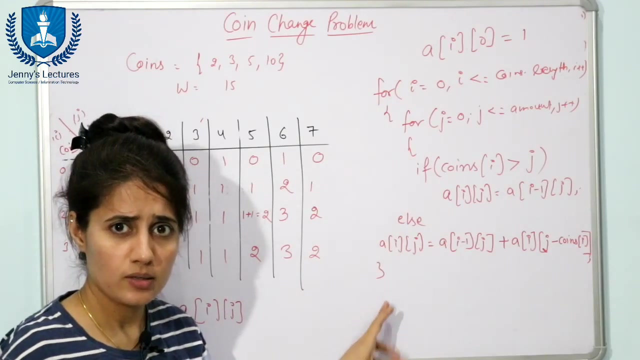 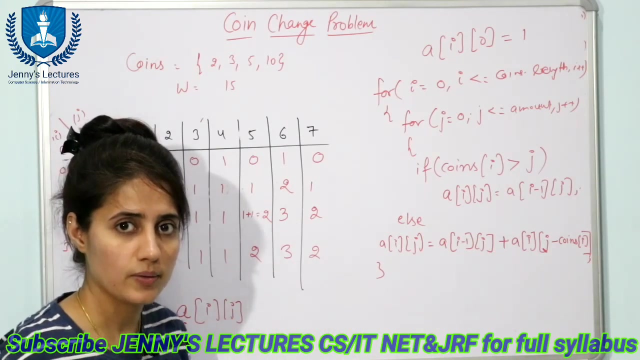 J Minus Coins. I, Because Coins Is This Name Of Array And I Value Is Here 2.. So This Is The Complete And Exact Program. 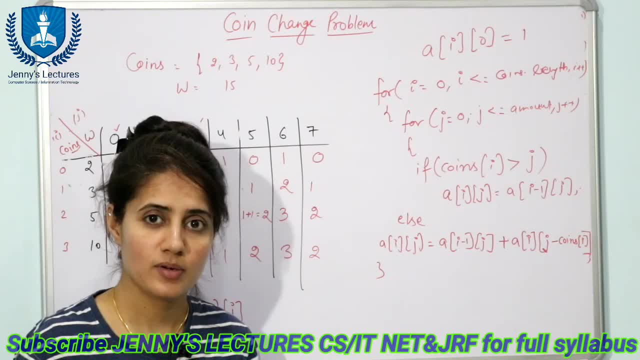 But This Is Somewhat The Logic You Will Write When You Will Code This Thing. Ok, So In Next Video I